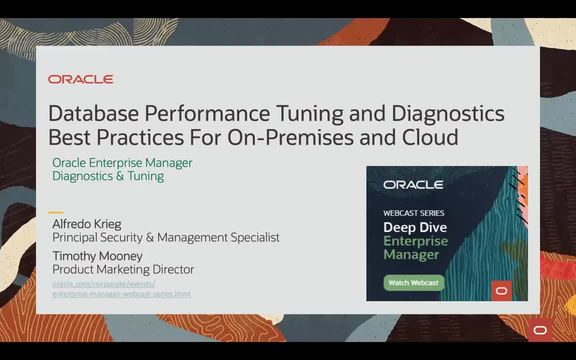 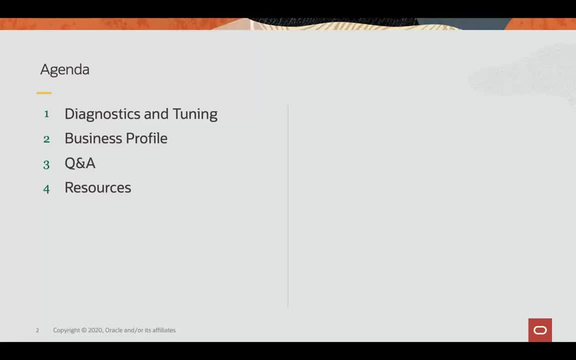 Definitely a deep dive. We'll go into diagnostics and tuning of databases. Alfredo will take you through an overview as well as some actual demonstrations using enterprise manager tools. Once he's done, I'll give you a quick business profile. We'll show some of the monetary benefits. 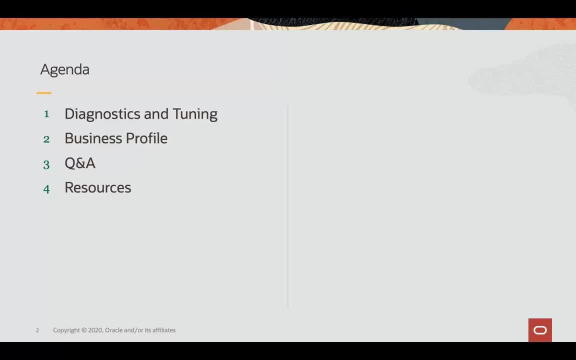 the business benefits of using enterprise manager. And then, most importantly, we have Q&A. We will have a little dedicated time at the end, but use that Q&A tab throughout our session. We're running this session for you guys And I think it's proven to be very valuable to leverage. 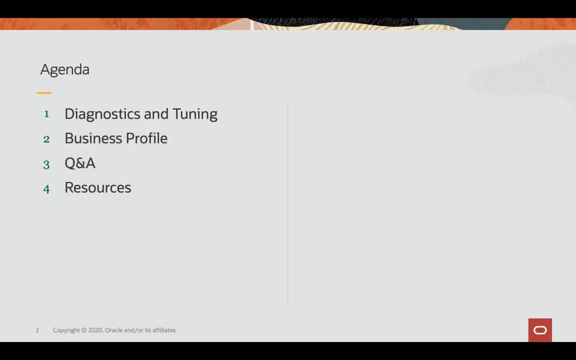 our experts ask your questions in that Q&A channel. If we can't get to them during the session, we'll be able to follow up with you And then we'll do a quick wrap with some additional resources and we'll be done So with that. let me turn it over to you. 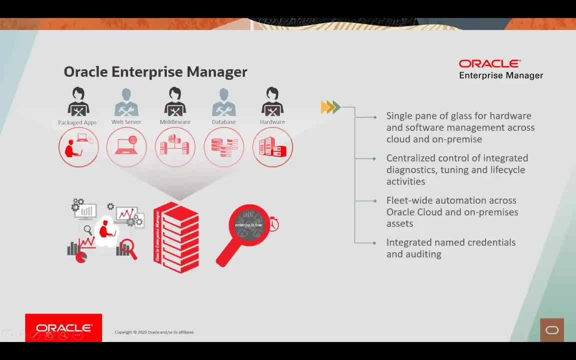 Alfredo. Thank you, Tim. Good morning, Good afternoon, Good evening everyone. Let's get started with this presentation about database performance tuning and diagnostics: best practices for on-premises and cloud infrastructure. We know that Oracle Enterprise Manager is Oracle's integrated 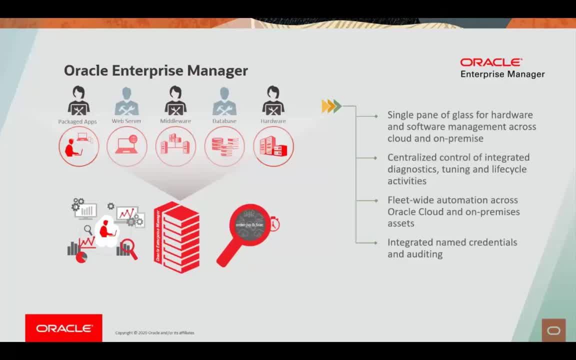 enterprise information technology management product line, which provides the industry's only complete, integrated and business-driven enterprise cloud management solution. Oracle Enterprise Manager provides a single pane of glass for hardware and software management across cloud and on-premises targets. It also provides a centralized control of integrated diagnostics, tuning and lifecycle. 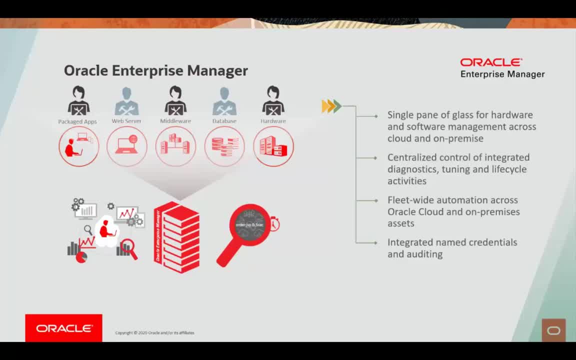 activities. The fleet-wide automation across Oracle Cloud and on-premises assets process helps us to achieve the best performance and the best performance for all of our customers, And that movements on-premises and amps our audit performance level to a slice thinking everything in their each-and-o-half-year system across theI10.. 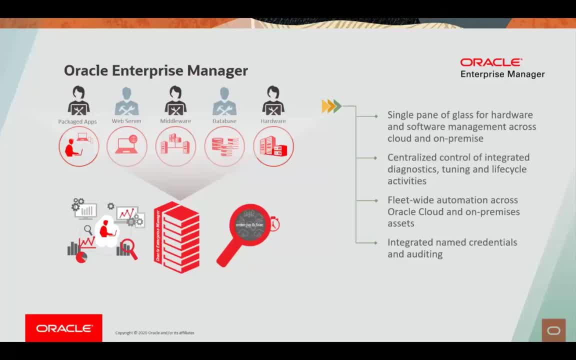 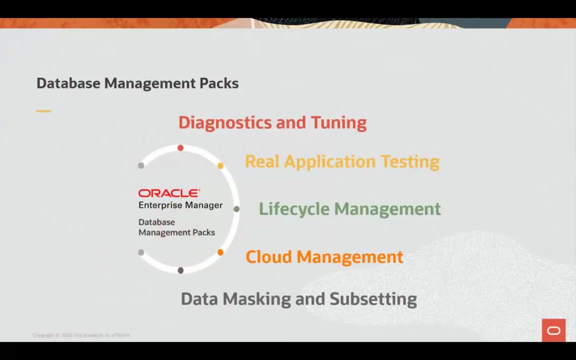 We straight away responded to this decision with URL on-premises. Oracle has been able to to target up to sweat um packs for the Oracle database, And all these packs, combined with Oracle Enterprise Manager's console and framework, help and allow administrators to better integrate solutions for diagnostics and tuning. 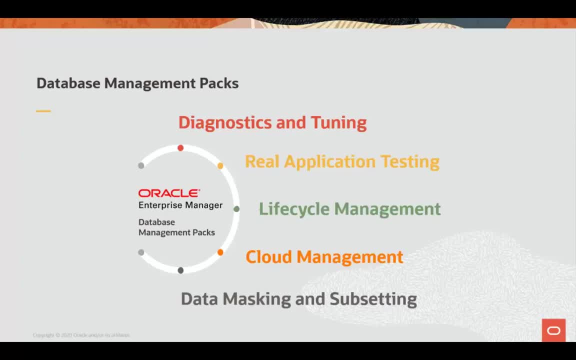 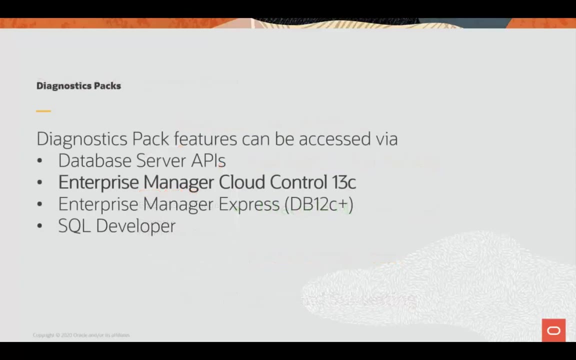 real application testing. also database lifecycle management activities, the database cloud management pack and, of course, data masking and subsetting. All these diagnostics packs can be accessed via either database server APIs using, of course, the Oracle Enterprise Manager Cloud Control 13c. 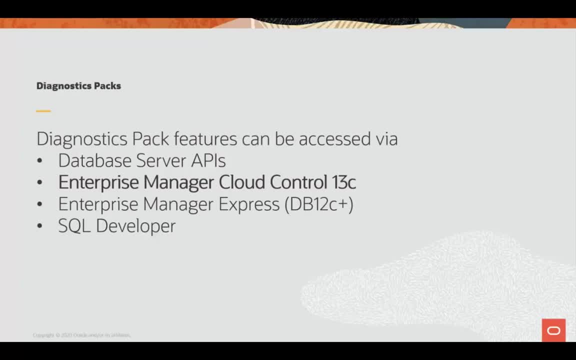 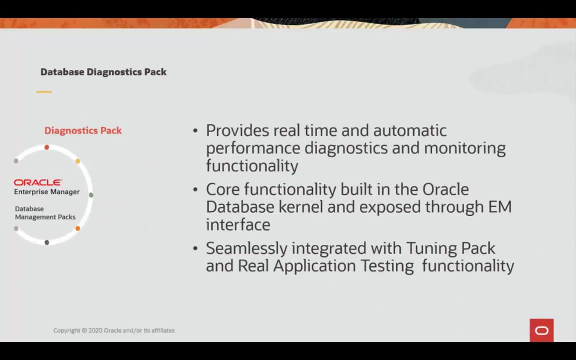 But also some of them can be accessed by using Enterprise Manager Express. This is available on database 12c And higher versions. Also, some of the features can be accessed using SQL Developer. Let's get started with the database diagnostics pack. 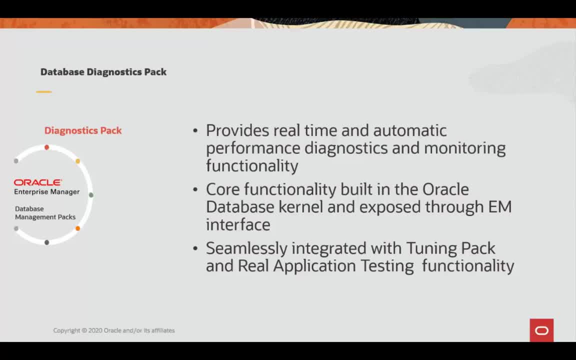 The database diagnostics pack provides real time and automatic performance diagnostics and monitoring functionality for your Oracle database. All this core functionality of the database diagnostics pack is built in in the Oracle database kernel And, of course, it's exposed through Oracle Enterprise Manager Interface. It's also seamlessly integrated with the tuning pack. 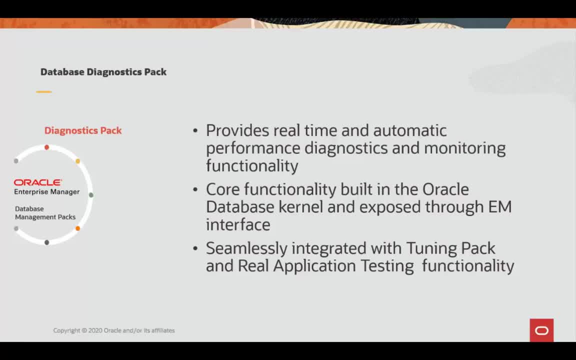 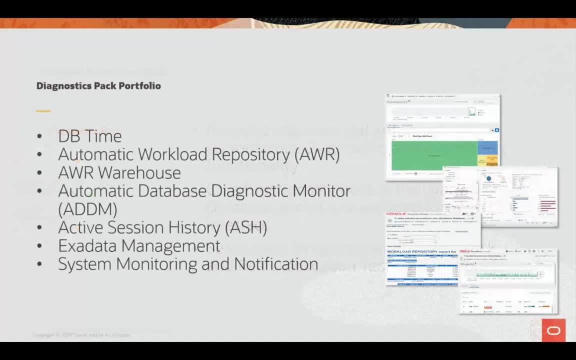 and real application testing functionality, And we're going to be covering that in future slides. The database diagnostics pack has a portfolio of tools inside which we're going to be covering here. the first one is, of course, the concept of using DB time. DB time is nothing more than the total workload. 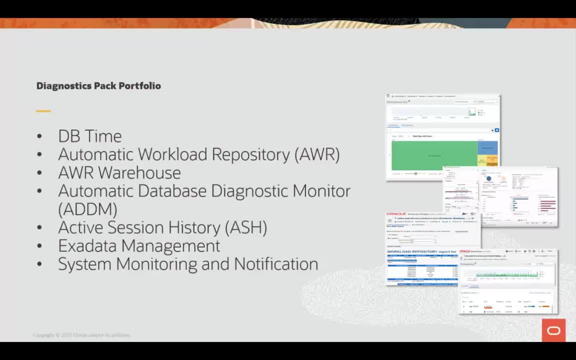 that the database is performing during a period of time. right, we also have the automatic workload repository- we call it AWR- and inside this automatic workload repository is where this kernel code is storing all this performance data that is gathering. then we make use of this AWR repository and all the views that 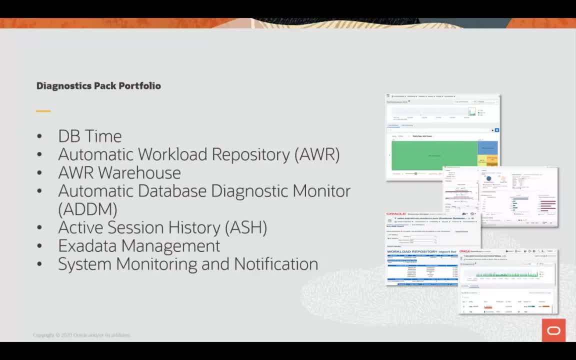 AWR is supposing to understand how the performance was in the past and we can start comparing actual performance with performance. that happened probably last week, yesterday or the day before, and then that helps you understand what changed in the database. we're also here. we're gonna be covering the AWR warehouse. we have the automatic database. 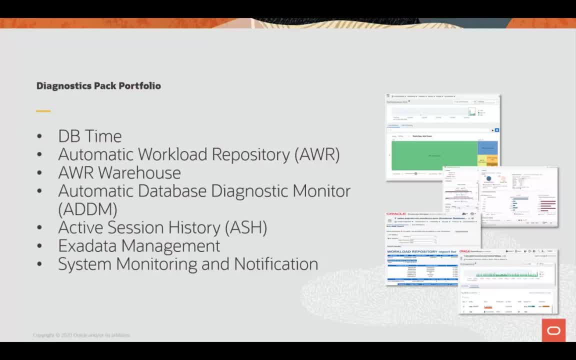 diagnostic monitor. we call it ADDM. another cool feature of the diagnostics pack is active session history ash. we have all the extra data management that is covered inside the diagnostics pack. that means when you discover and you manage and monitor your exit data, you require the diagnostics pack in order to do that. and, last but not least, we have the system. 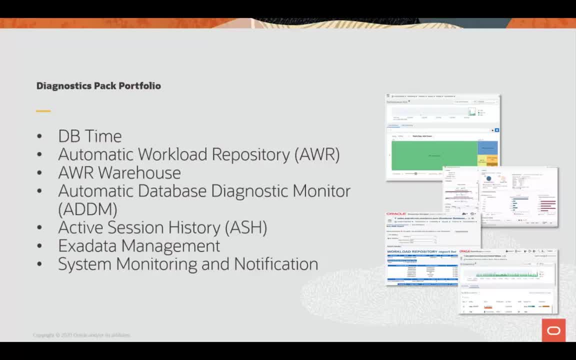 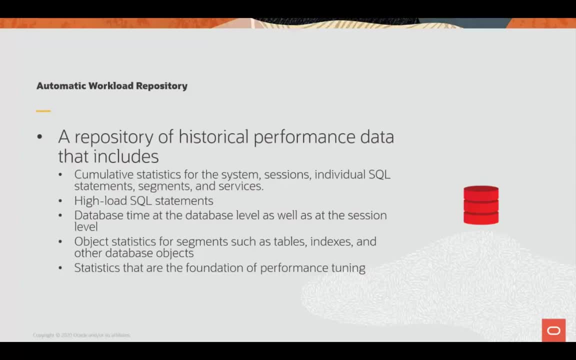 monitoring and notification system. as I mentioned, the automatic workload repository is a repository of historical performance data. all this performance data is being gathered by the database itself and is stored inside a table space in your database. All this data includes cumulative statistics for the system, for the sessions and also 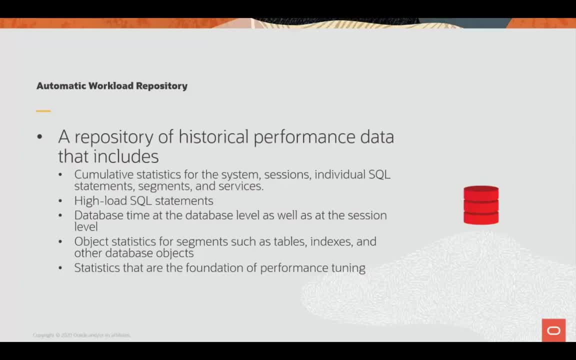 individual SQL statements, segments and services. It also includes high load SQL statements. It includes the concept of the database time at the database level and as well as the session level, So you can start comparing and gathering information about the amount of workload that the database. 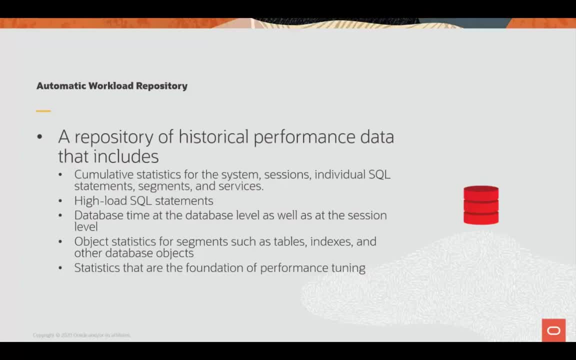 is processing, either at the database level as a whole or at the session level. We also have object statistics for segments such as tables, indexes and other database objects. These statistics are the foundation of performance learning. Without this data, it will be really difficult for us to go back in time and understand how. 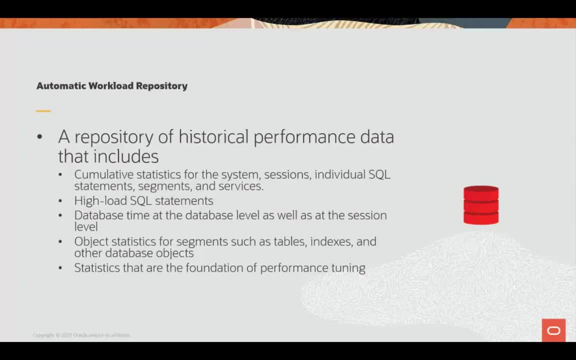 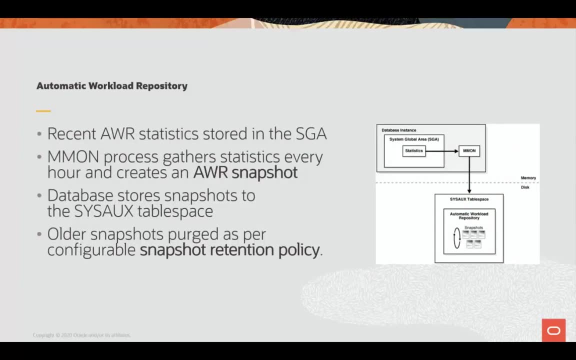 was the performance before the issue that we're facing right now in the database, right? So how this works, as you can see in this slide, we have in the right side we have the database instance. The database instance is comprised of memory area, pools and processes, right. 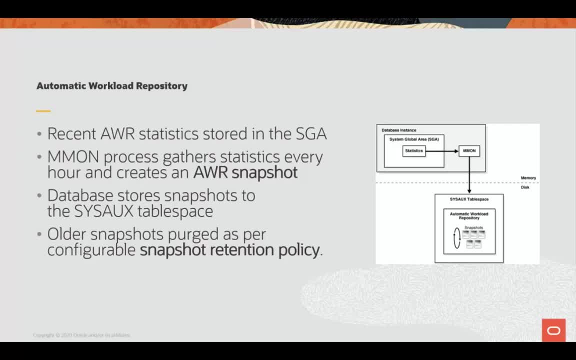 Inside the kernel code we have instrumentation of the database. That instrumentation, what it's doing is gathering all these statistics and it's storing those statistics in the SGA- okay, because it's a memory pool in your server. Then we have a background process named MMO. 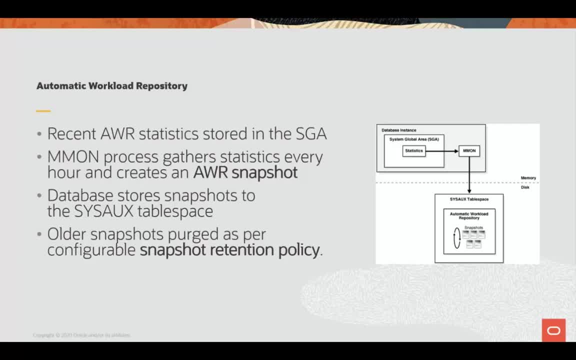 That is going to gather these statistics every hour and it's going to create an AWR snapshot. An AWR snapshot is nothing more than a picture of your database at a given time. right, We're going to be storing that inside the AWR repository. 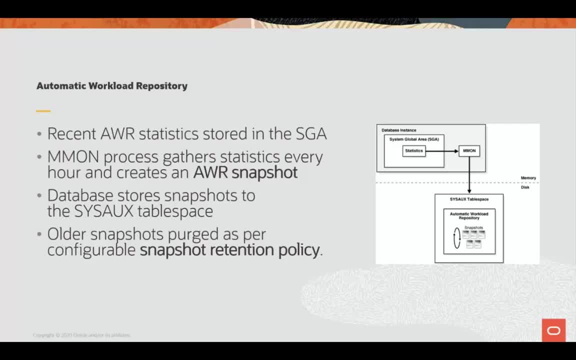 The database is going to store these snapshots, these pictures of the database, inside a table space named SISOX, okay, And of course we have rotation and we have maintenance of this information And these older snapshots are purged as this configurable snapshot retention policy. 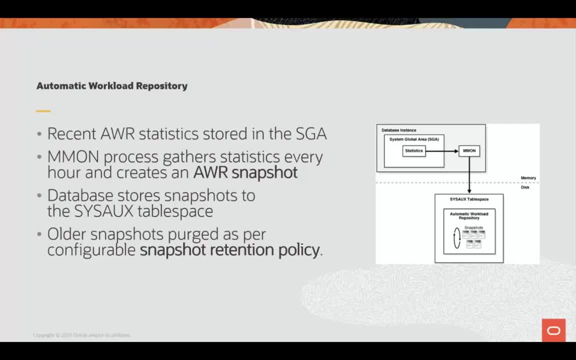 That means that you can go back and instruct the database and say how much data you want to store in that particular AWR repository. By default we have eight days. Okay, Our recommendation is to modify that accordingly to your business needs, right? 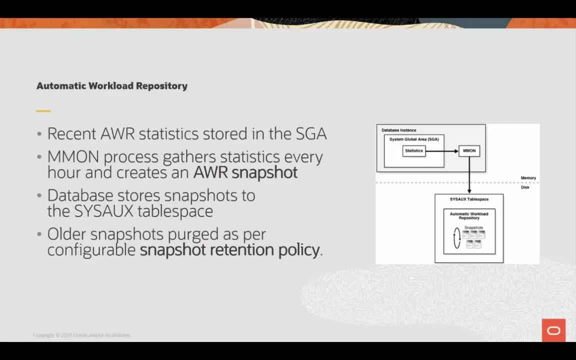 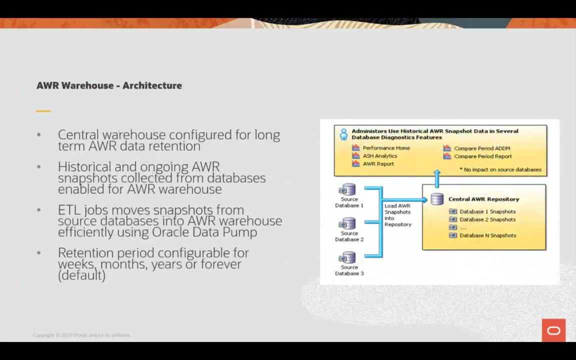 Keep in mind that the more data you store, the bigger the SISOX table space is going to get. So now that takes me to the concept of AWR Warehouse, And AWR Warehouse is a central warehouse That you can configure for long-term AWR data retention. 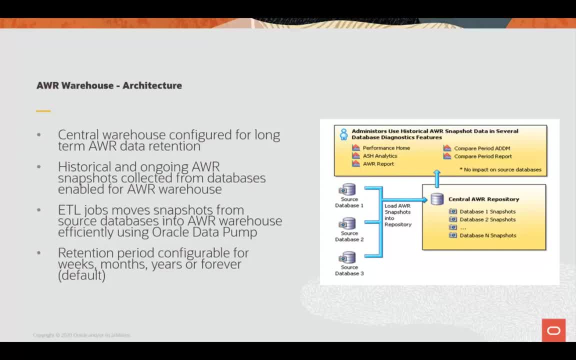 In my previous slide I mentioned that the more data you store, the bigger that SISOX table space is going to get right. So what happens when you start gathering snapshots, let's say every 5, 10 minutes, because that's. 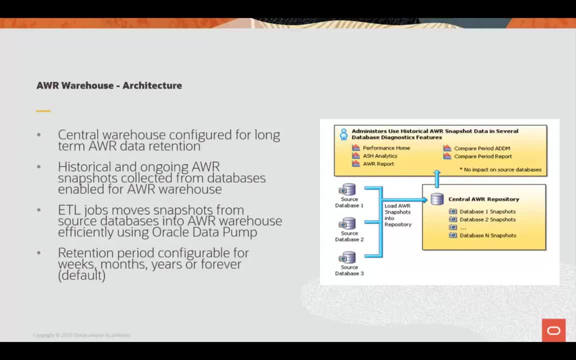 what your business is in need of And your retention policy is, let's say, 180 days, that you're required to store that performance data. You are required to go back in time and compare the performance back to 180 days, right? 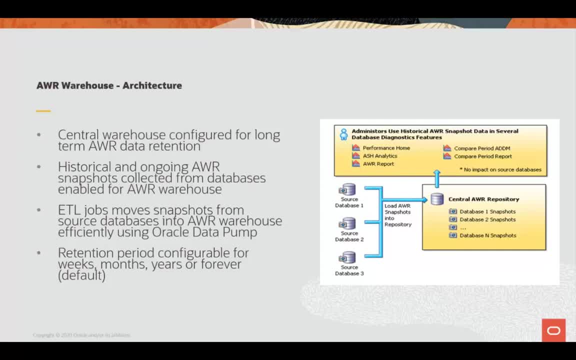 That SISOX table space is going to grow big. That brings several challenges right. The first one that comes to my mind is backups. You're going to be backing up this data. Your backups are going to be getting bigger as well. 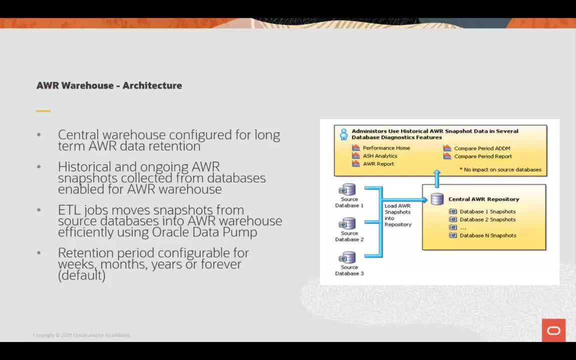 When you clone databases- let's say, you have a requirement to clone this production database to test dev or QA environments- then you're cloning this data along with, So you are using more and more data for your clone databases, right? So in order to overcome this, inside Oracle Enterprise Manager, we have this AWR Warehouse. 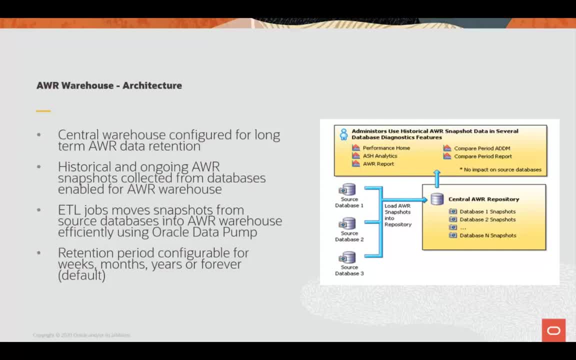 functionality. That means that you create an additional Oracle database that is going to serve as an AWR Warehouse repository And then you configure Enterprise Manager. As you can see, you instruct Enterprise Manager which ones are going to be your source databases. These source databases are going to be configured in Enterprise Manager. 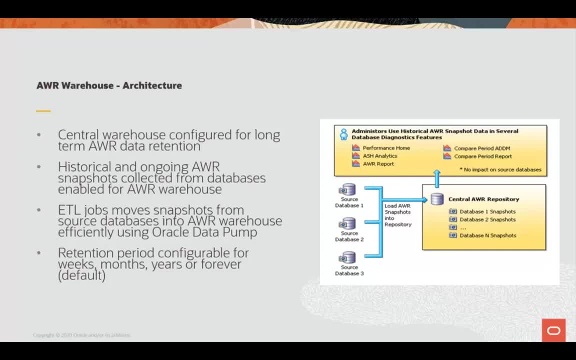 And Enterprise Manager has ETL jobs. These ETL jobs, their functionality, is to go to these source databases, extract this AWR data and import the data into your AWR Warehouse. This is using Oracle Data Pump in the background, right. 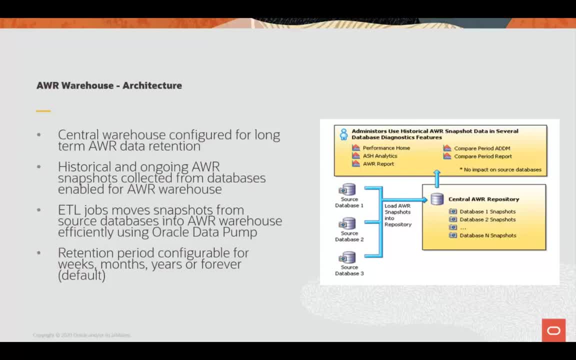 And last but not least, you can configure the retention period for this AWR Warehouse. By default, it's forever, Right, That means that you can store this data forever. You can go back in time. let's say: how was the performance of this production database? 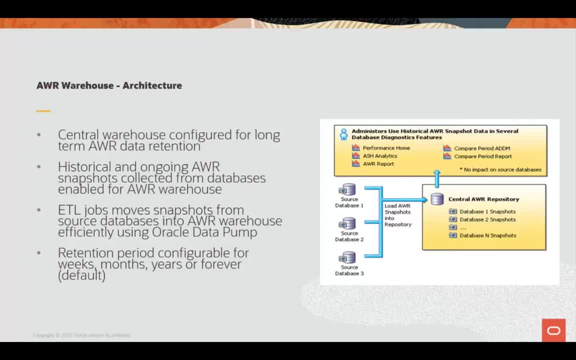 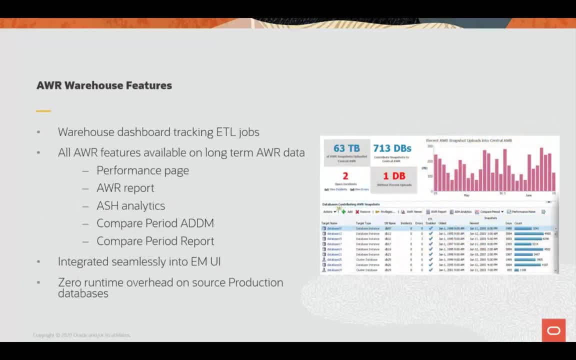 two years ago. right, It's a useful feature for Oracle database administrators. So this is a screenshot of an AWR Warehouse dashboard. As you can see, we have an AWR Warehouse dashboard And then you can see a screenshot of the dashboard. 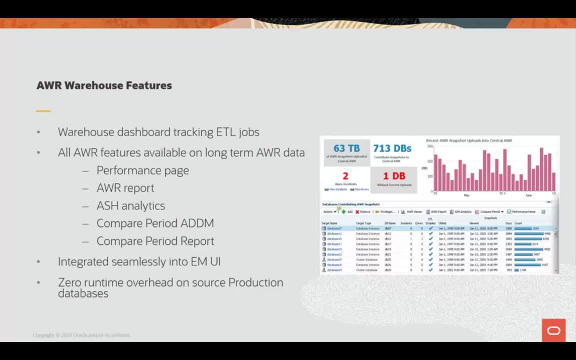 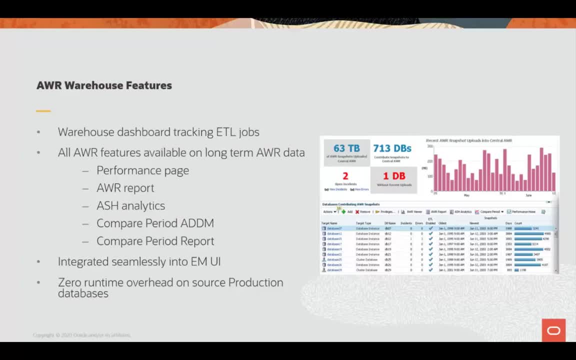 So on the lower part of the snapshot you can see that we have our target databases, the target types, the database names, if the ETL jobs are enabled or not, if there are any incidents, any errors in extracting that AWR data, and how many days we have worth of AWR data for each of the databases right? 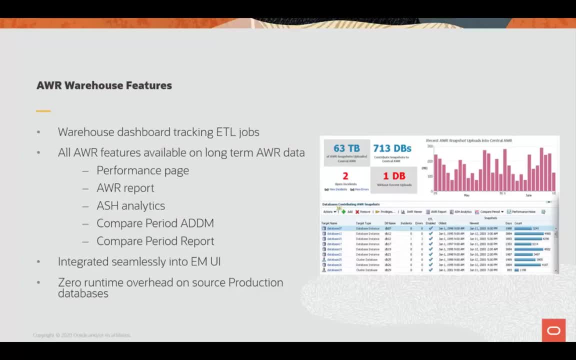 You can also use. You can use this performance page to understand how much data you're loading, how much data you're generating, And from here you can create AWR reports. You can call Azure Analytics to find out how the performance is. 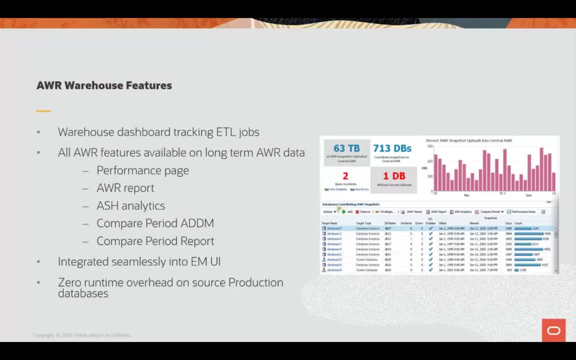 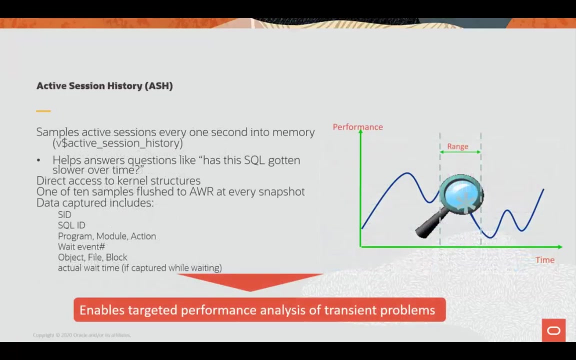 You can also execute compare period ADDM reports and also compare period AWR reports. As you can see, this is integrated seamlessly into the Oracle Enterprise Manager UI And it's zero runtime overhead on the source production database. when we extract the data, We have also active session history, ASH. 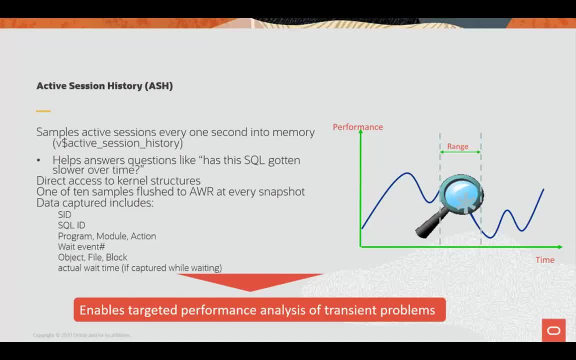 The way ASH works is: we're going to be sampling active sessions- And I quote again, active sessions. This is an important concept- Every one second. We're going to be sampling data into memory And you can query this data by using the system. view V-dollar active session history. right, 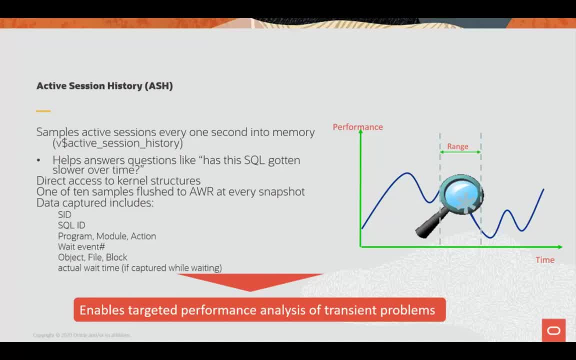 Active session history helps to answer a couple of questions like: has this SQL gotten slower over time, right? Active session history has direct access to kernel structures. That means that the kernel code of the database is the one that is responsible of this sampling, And one of 10 samples are flushed to AWR at every snapshot that we take. 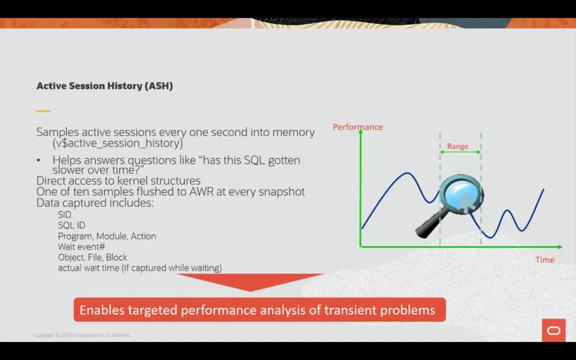 That means that you have to keep in mind that this is not 100% accurate data. This is a sampling, But it's good enough to understand how the active sessions are performing in our database system. Some of the data that is captured Includes the SID. 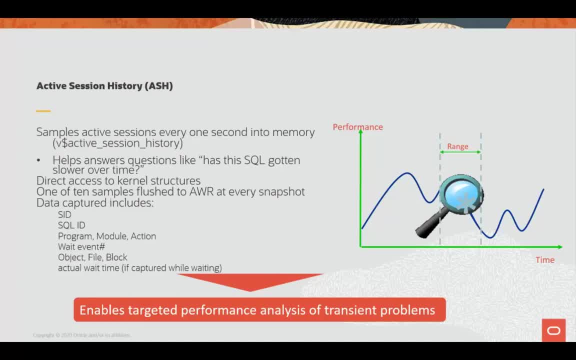 Of course, the SQL ID that is executing right, The program, the module and the action. We also have the wait event number and also the object, the file, the block and the actual wait time, If, when we're capturing that session is waiting right. 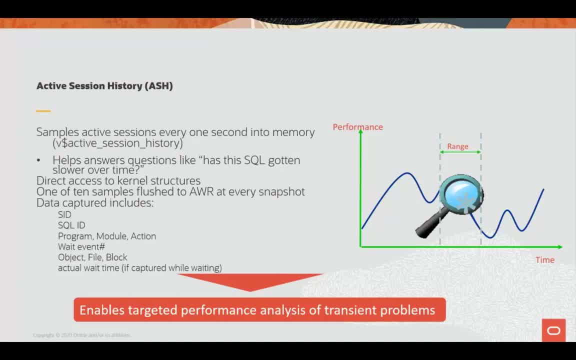 All this information enables the administrator to have a target performance. All this information enables the administrator to have a target performance And the analysis for transit problems in the database. That means that you can define a range where you want to get that active session history report. 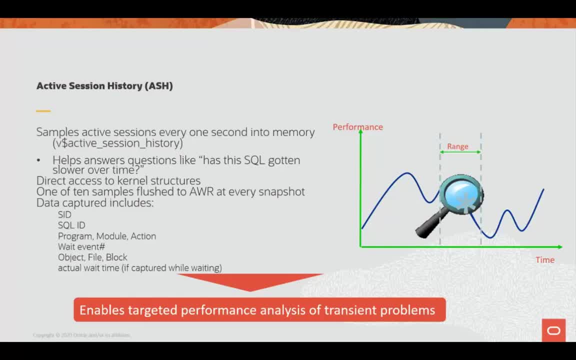 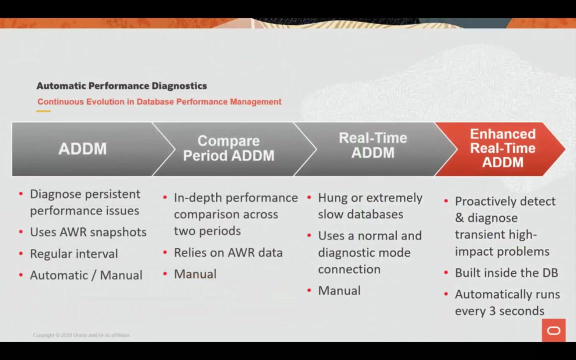 You can also filter by wait event. So you can say: I want to filter during this period of time of the sessions waiting on this particular wait class, right. So it's really important tool When we're troubleshooting performance issues. Moving forward, we have the automatic performance diagnostics. 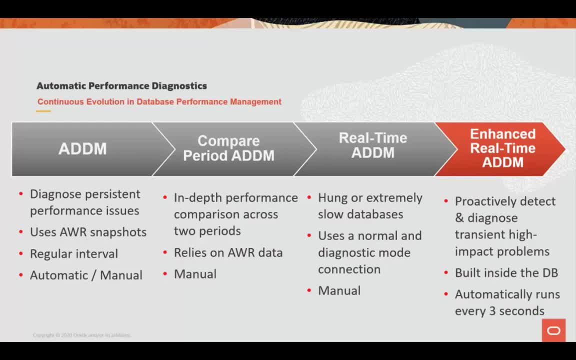 And this is the way we call it- is the continuous evolution in database performance management. So ADDM help us to diagnose persistent performance issues. It also make use of AWR snapshots, So at the end we're going back to the basics, Where 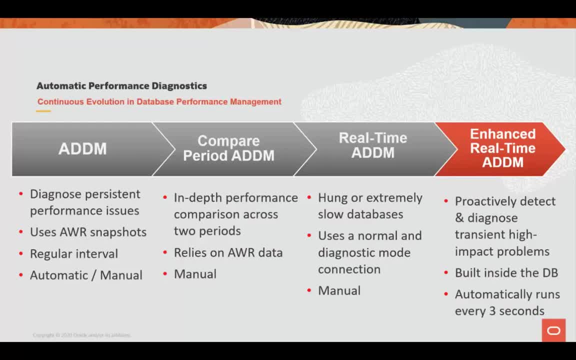 ADDM helps us to diagnose persistent performance issues. It also make use of AWR snapshots. Without AWR data, we will not be able to understand the database performance. This ADDM can run at a regular interval And you can configure ADDM to run either automatic or manual right. 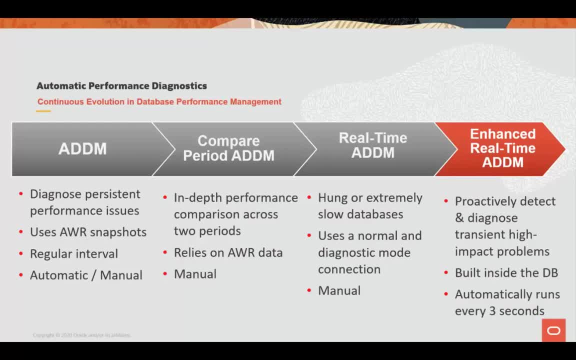 We also have the option to run a compare period, ADDM. that is going to provide us in depth performance comparison across two periods. That means that we get- we instruct ADDM to get- one snapshot and compare that against a different snapshot. Again, it relies on AWR data and this is a manual task that you have to manually start, okay. 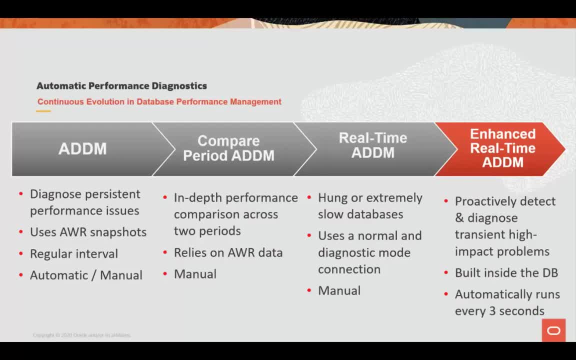 We have also real-time ADDM and that help us to understand why a database is extremely slow or when the database is hung, That means that you're not able to connect to the database. It uses a normal, but also has the ability to connect to the database in diagnostic mode. 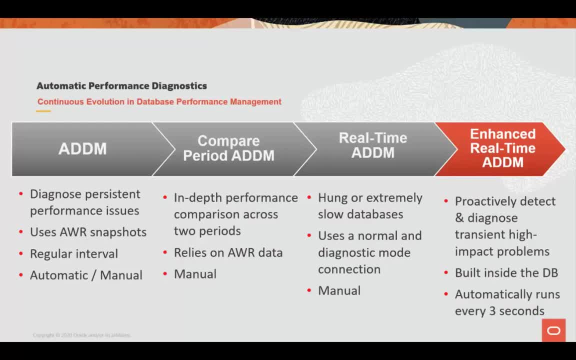 That means that we have a backdoor in the database where we allow ADDM to connect and provide you information on what's happening in the database. when you're not able to connect normally This one, you have to start it manually, and I'll show you some of the screenshots that we have. 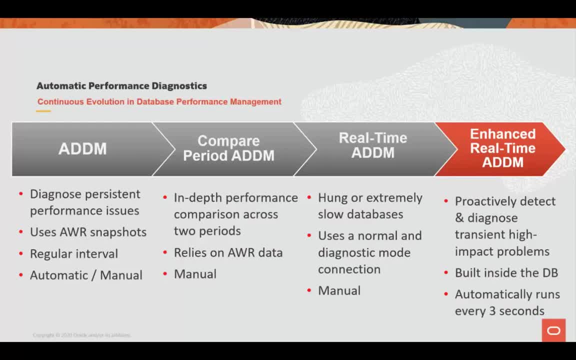 for real-time. I'll show you some of the screenshots that we have for real-time ADDM just in a minute. Last but not least, we have the enhanced real-time ADDM, which, proactively, is going to detect and diagnose transient high-input problems. 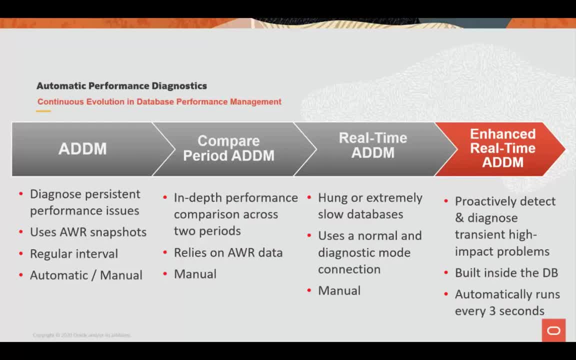 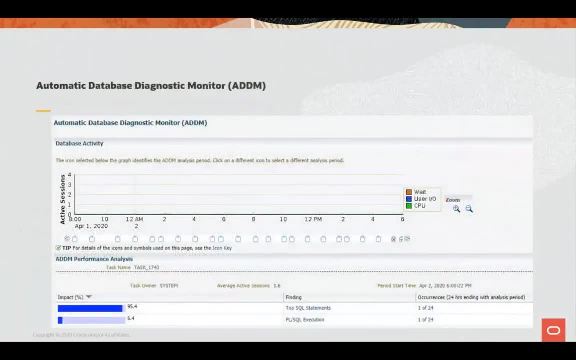 This one is built inside database and is running automatically every three seconds For the automatic database diagnostic monitor, the standard ADDM. you can see that we have a chart with a timeframe of snapshots. These are the available snapshots that we have in our database in our AWR repository. 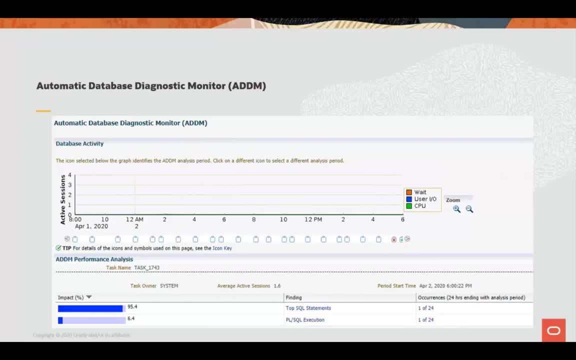 And then you will have to select which one is going to be the beginning and the end snapshot. You instruct ADDM and it's going to produce a report. You can see in the lower part of the screenshot that there is an impact of 95% and the finding is top SQL statements. 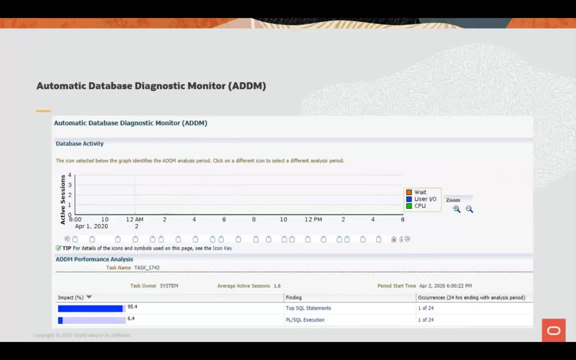 That means that ADDM is finding that some SQL statements have an impact in the performance database of around 95%. okay, You can click on that finding and it's going to give you a detailed information of which SQL statements are the ones that are consuming or have. 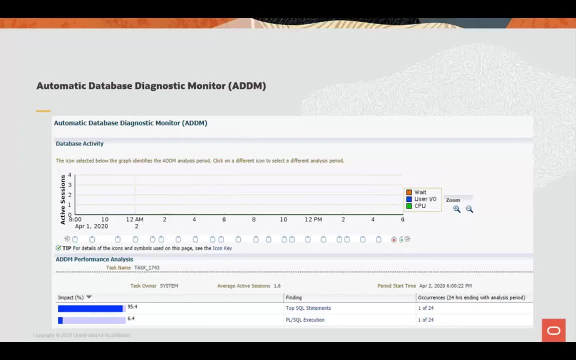 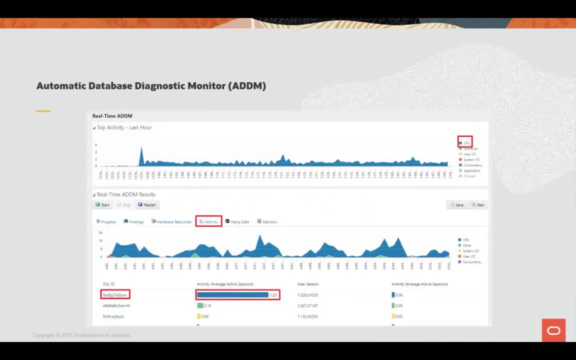 higher impact in the database performance For real-time ADDM. we have the top activity graph. You can see that this is for the last hour. right On the middle screen you can see three buttons. The first one is a start. That means that. 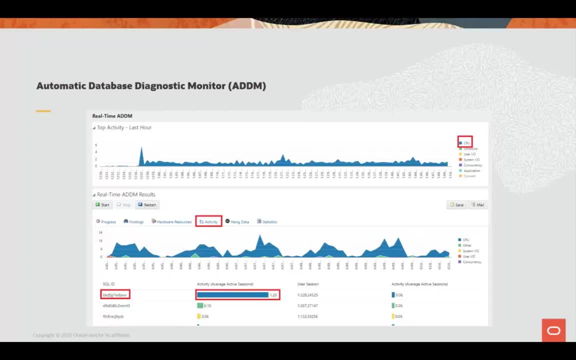 you have to manually go and click start in order to initiate the process of connecting to the database. You can stop that process or you can restart that connection. Then, when ADDM is done, gathering all the needed information, it's gonna produce that report that I'm showing you here. So I 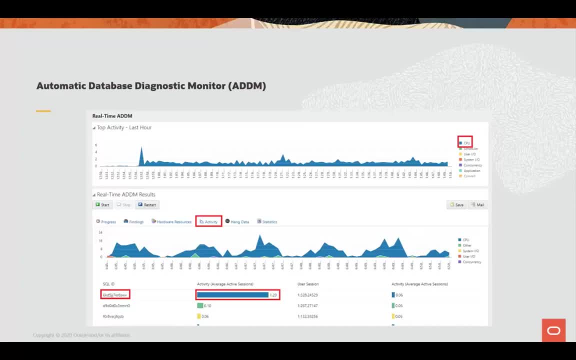 click on activity, You can see that there is a SQL ID that is highlighted in red and also the activity of that particular SQL ID is giving you this user session information and also the activity in average active sessions. right, We have also a graph that is showing you which weight classes are the ones that 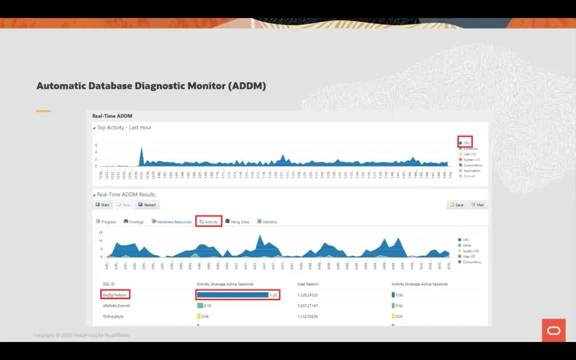 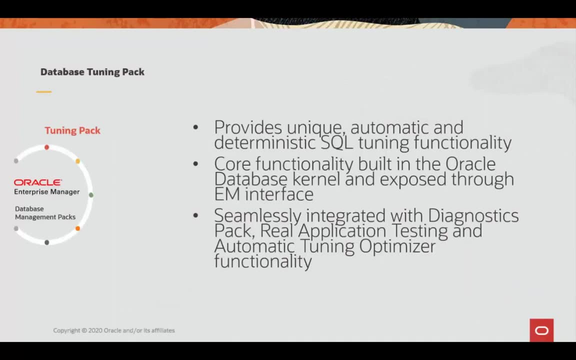 are consuming more resources in your database. In this example, we have that most of our sessions are consuming CPU. The database stunning pack provides a unique automatic and deterministic SQL tuning functionality. okay, All this functionality is also built in inside the Oracle database kernel and the. 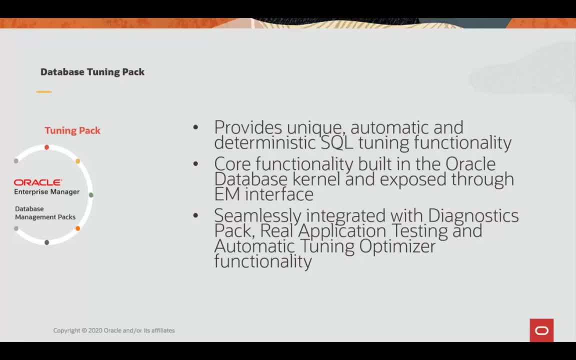 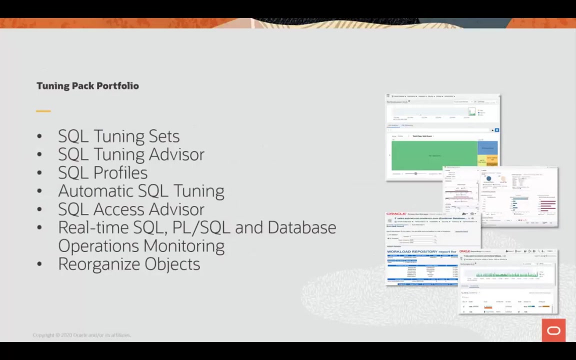 same way as the database diagnostics pack is exposed through the Oracle Enterprise Manager interface, It's also integrated with the diagnostics pack the real application testing and automatic tuning optimizer functionality. So some of the tools inside the database stunning pack are SQL tuning sets. We have 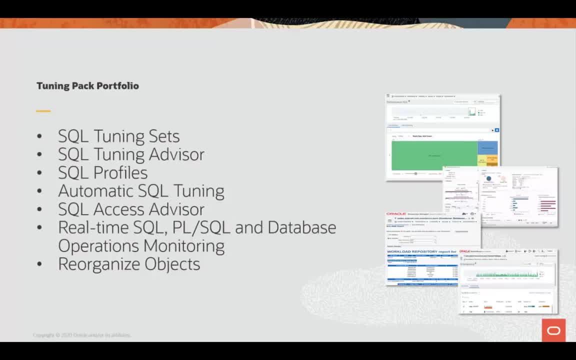 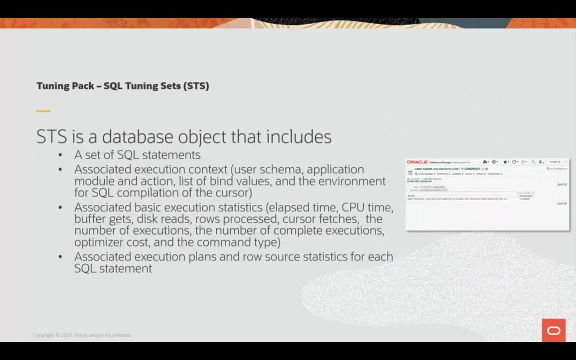 the SQL Tuning Advisor. We have SQL profiles, the automatic SQL tuning, SQL Access Advisor, We have real-time SQL, PL SQL and database operations and monitoring and we also have the ability to reorganize objects. So a SQL turning set, A SQL turning set- is a database object. This SQL turning set includes: 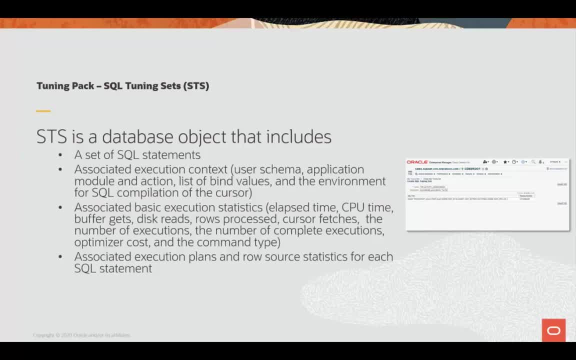 a set of SQL statements. It can include one or multiple SQL statements. That means that we can call it a container of SQL statements. It also contains all the associated execution contexts. That means the user schema, the application module, the action, If it has. 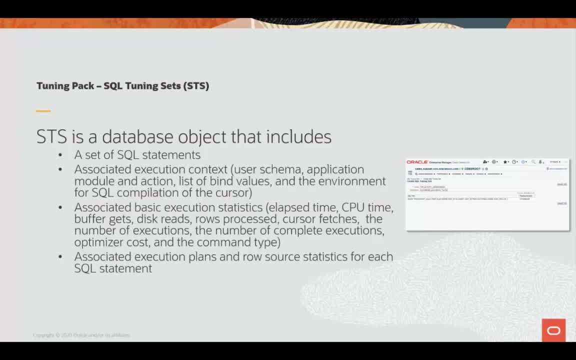 any bind values. all the bind values are inside the SQL turning set And also the environment for the SQL compilation of the cursor. All the information of the cursor is inside the SQL turning set. It also has all the associated basic execution statistics. means elapsed time. CPU time buffer gets disk reads the number of rows processed. 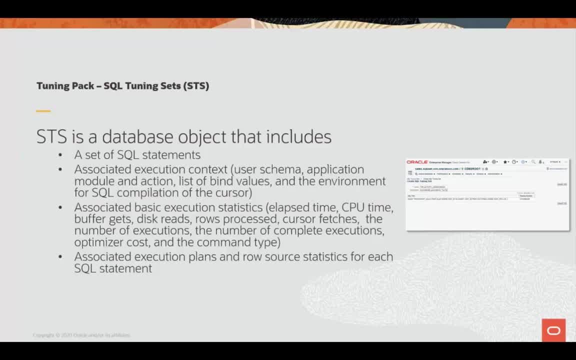 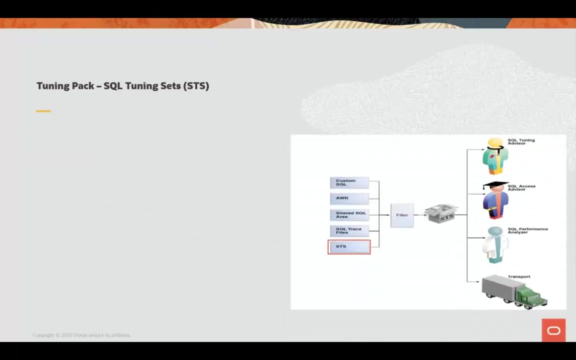 how many cursor fetches that SQL statement had to execute, the number of executions, the number of complete executions, the optimizer cost and the command type that was used. All the execution plans and the row source statistics are also included inside the SQL toning set. 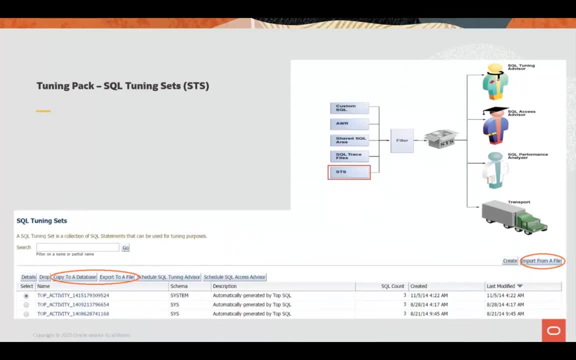 We can also make use of Oracle Enterprise Manager to create SQL toning sets. We can click the button Create, We specify a time frame where Oracle Enterprise Manager is going to start capturing SQLs and it's going to be starting, Okay, So we can start storing those SQL statements inside that particular toning set, right. 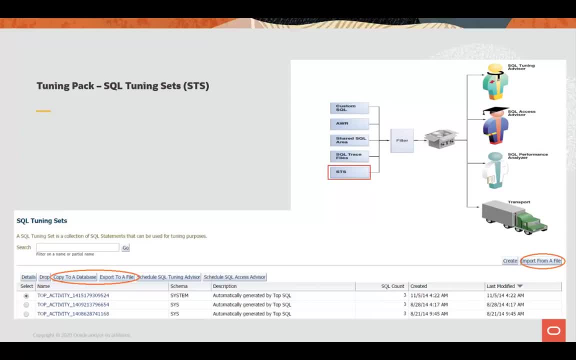 You can filter SQLs. It has different advanced filtering options for you. You can transfer these SQL toning sets between databases And the idea is, if you're troubleshooting an issue on a production database, you can go ahead and create a SQL toning set. 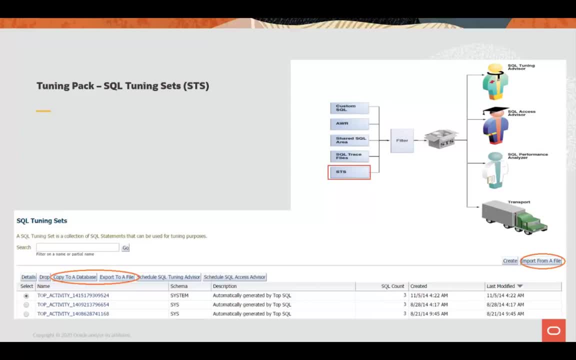 that contains SQL toning sets. It contains the SQL statements that you're interested in and fix. Then you transfer that SQL toning set to a test environment that is similar to that production database And then you can start doing the troubleshooting or modifying those SQL statements. 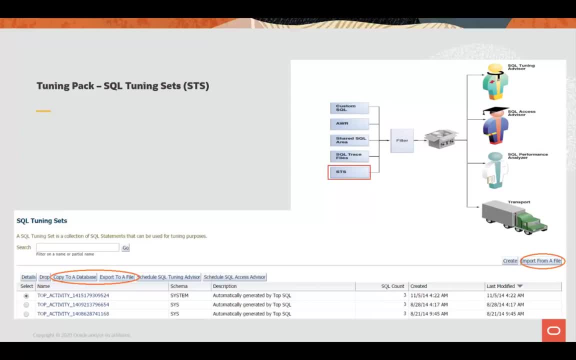 in that test environment without affecting production The way you transfer that. you can go and manually execute commands. But if you use Oracle Enterprise Manager, you can click on that Copy to a Database button. Basically what you require is a directory object that was created in that database. 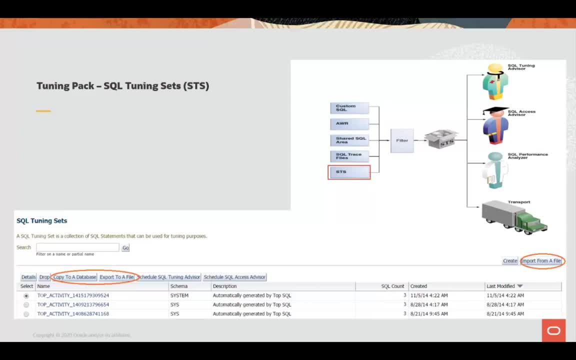 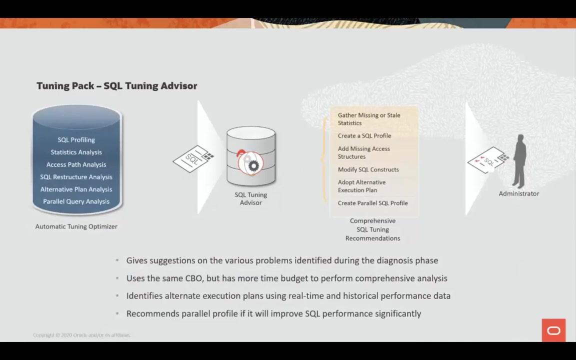 Oracle Enterprise Manager is going to run behind scenes all the exporting and importing for you. If you want to do it manually, you can also click on Export to a File and then you can import from a file inside the test database. This L earn saving for other different apps and different objects as you move to buyers, function and 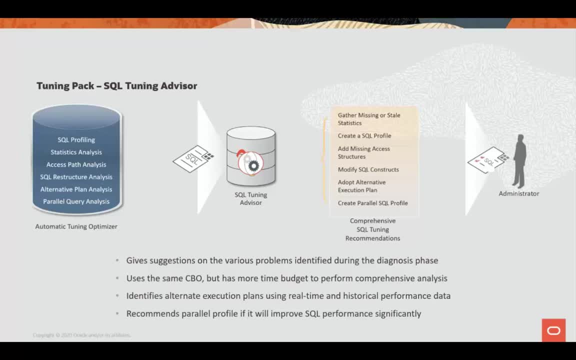 license, Or you can also change from편 the device to sliding CHRIST. Let's move now forward to SQL Toning Advisor. The SQL Toning Advisor is going to give you suggestions on the problems that were identified during the diagnosis phase. That means that you have to instruct SQL Toning Advisor to start diagnosing SQL statements. 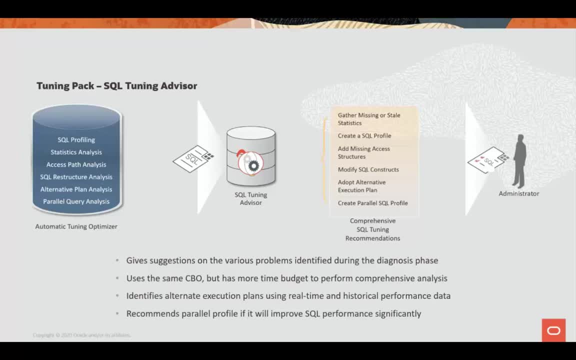 and analyze one SQL statement or multiple SQL statements by providing a SQL turning set right. he's gonna use in the background the same CBO, the cost-based optimizer, but has more time to budget. more time budget to perform comprehensive analysis. what this means when you are parsing a SQL statement. 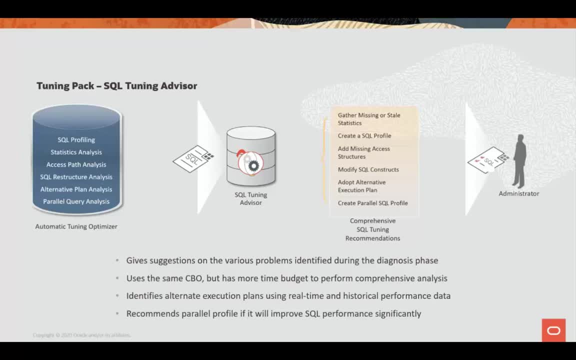 right, basically, what you're doing is you're passing the sequel text and then you instruct the database to generate an executable code inside the, the RDBMS, the, the cost base optimizer, has microseconds to identify multiple execution plans and then choose the best execution plan for that particular SQL statement. right, so? 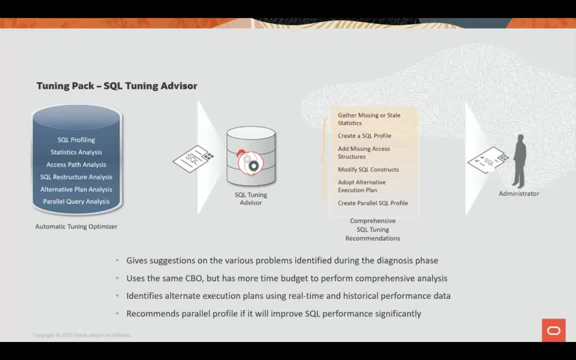 it has limited time during the parsing of the SQL statement- right, so it has limited time during the parsing of the SQL statement: right. so it has limited time during the parsing of operation. when you instruct the SQL turning advisor to analyze a SQL operation. when you instruct the SQL turning advisor to analyze a SQL. 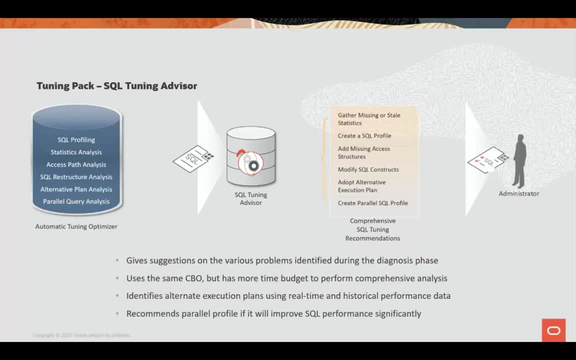 statement. then you can define that time frame that the SQL turning advisor has for that particular operation. by default is five minutes. so just imagine in five minutes how many execution paths can the the CBO find for that particular SQL statement. that means that has more time to analyze more paths and give you a 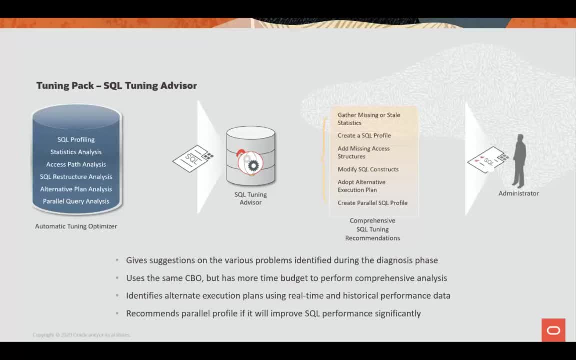 better execution plan for that particular SQL statement, right, so it's better execution plan for that particular SQL statement, right, so it's again. SQL turning advisor is going to identify these alternate execution plans using the real-time and historical performance data that we already have inside AWR, and it's going to recommend SQL profiles, or it's going to recommend. 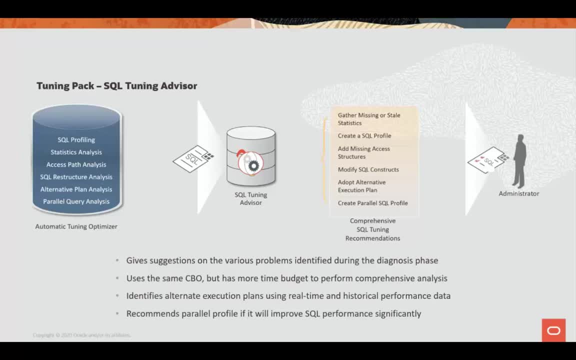 gathering, missing all stairs statistics or adding missing access structures like an index, or create a materialized view, modify SQL constructs, adapt alternative execution plans or even create a parallel SQL profile if the CBO finds that running a parallel SQL is better than on the standard SQL statement, and then at the end it's up to the administrator to. 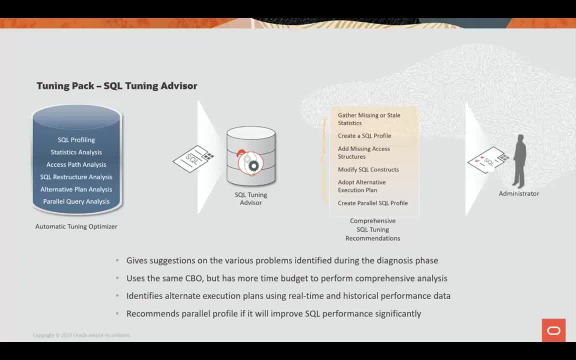 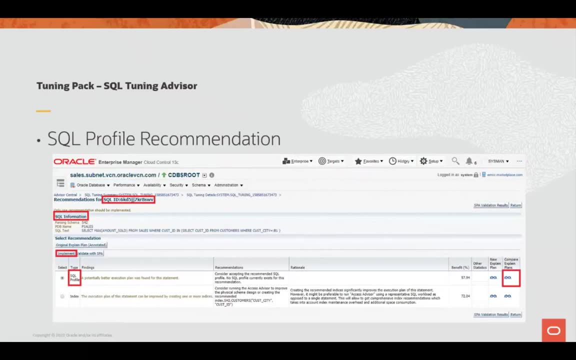 accept those recommendations inside the database. let me give you an example. so this is a dashboard of a recommendation that can be implemented in the SQL. out out of the the SQL training advisor, you can see that we have the SQL ID highlighted. we have the SQL information, so it's giving us information about the. 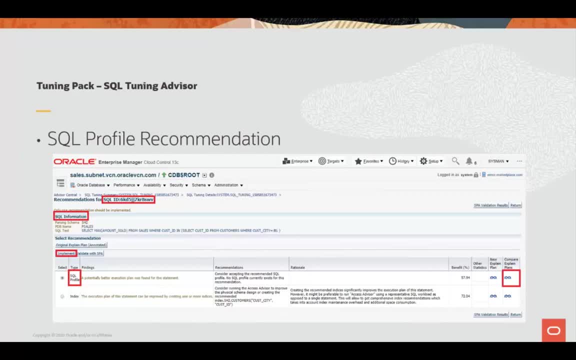 SQL text, the PDB name and the parsing schema. and then it has a table where is providing you the the recommendations after the analysis, right, so you can go ahead and click that compare, explain plan, for example, for for the first recommendation, which is a sequel profile, you can see that the benefit of 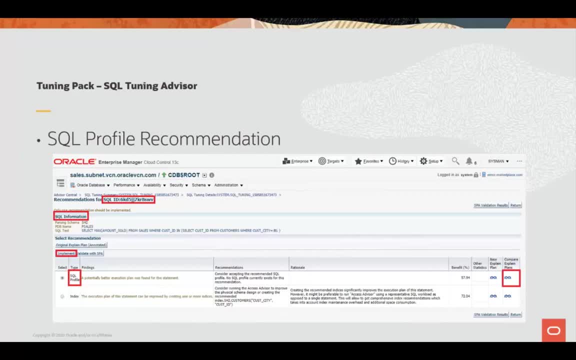 implementing that sequel profile is around 58%. you can click on compare explain plans and it was gonna provide you information of what is the- the previous, the original execution plan- compared with a new explain plan that is going to be created if you accept that sequel profile. the second recommendation is to create an index. right, it's giving you. 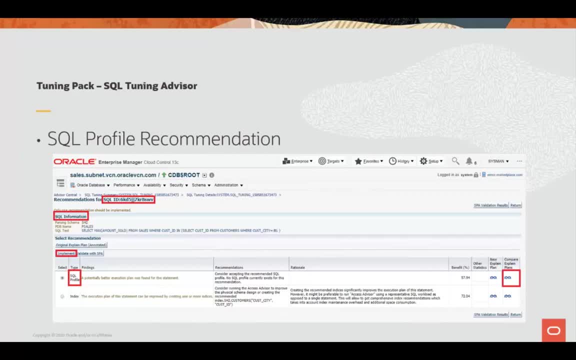 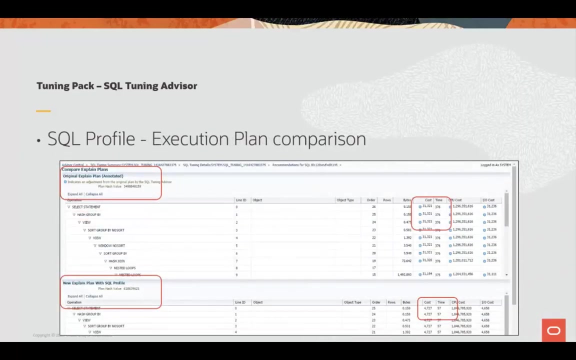 information about where it's gonna create that index. in this case is the customers table on the cost city and the cost ID columns right, the benefit around 72%. you can also see the new explain plan or you can compare this explain plans. if I click on compare explain plans for the SQL profile, I get a. 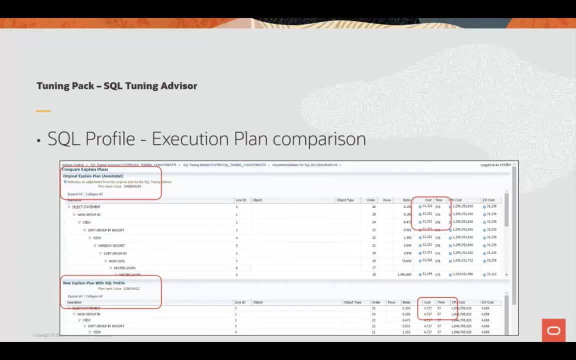 a, a a page like this one, the, the one that I'm showing you right now. this is the execution plan comparison. we have the compare explain plans. we have the original plan on the top along with the plan hash value, and also we have the new explain plan with a new hash value, and you can see the difference in the cost. 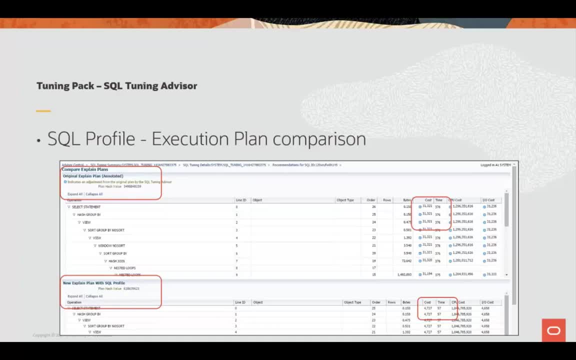 the original one is around 31,000. you can see the time is 376, compared with the cost of the new one, which is the cost of the new one, which is the cost of the new one, which is 47, 127 and the time is around 57. right, much better than the original. 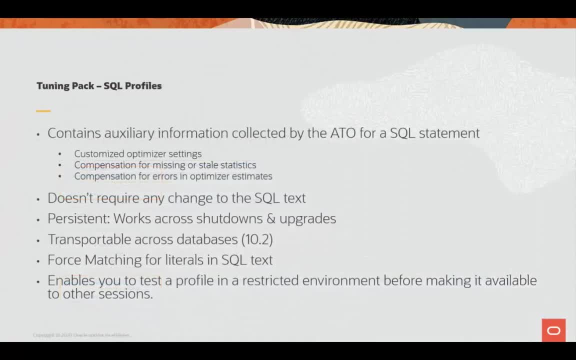 one. so when you create a sequel profile right out of the recommendation of the sequel turning advisor, well, what is? what is a sequel profile in database? a sequel profile is another database object. this sequel profile, as I mentioned, contains a. this is another database object. this sequel profile, as I mentioned, contains a. 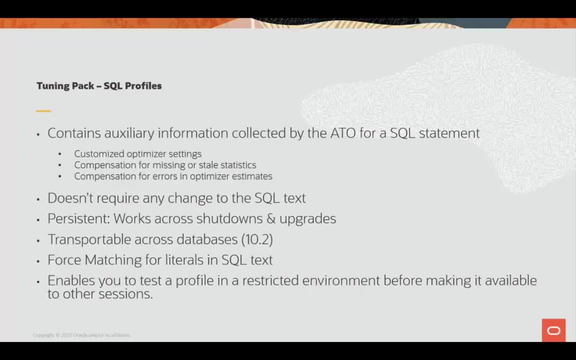 auxiliary information. this is collared, collected by the SQL turning advisor for auxiliary information. this is collared, collected by the SQL turning advisor for that particular sequel statement. it contains customized optimizer settings it that particular sequel statement. it contains customized optimizer settings. it also contains that compensation for missing or stale statistics or 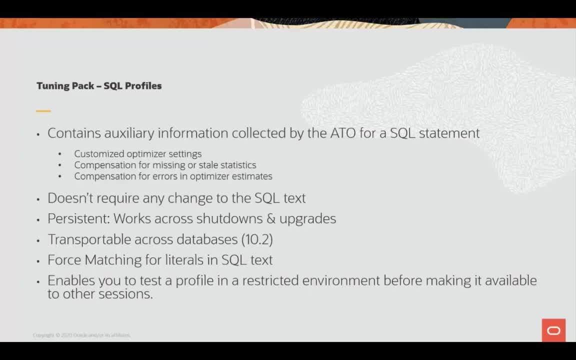 compensation for errors in optimizer estimates. it doesn't require any changes to the original sequel text. that means that you can implement that that inside your database without asking your developers to modify the SQL statement. It is persistent. That means that it works across shutdowns or upgrades. 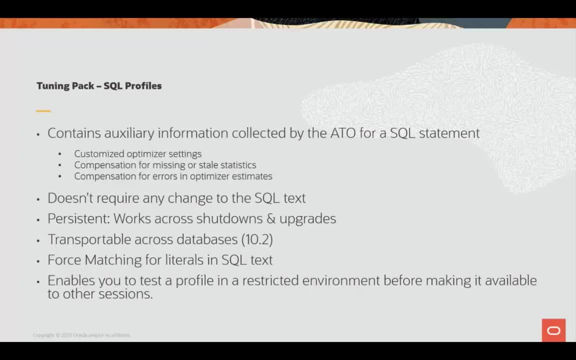 You can transport that across databases. This is functionality coming from 10.2 version of the database. You can force match option for literals in a SQL text And also this enables you to test a profile in a restricted environment before making it available to other sessions. 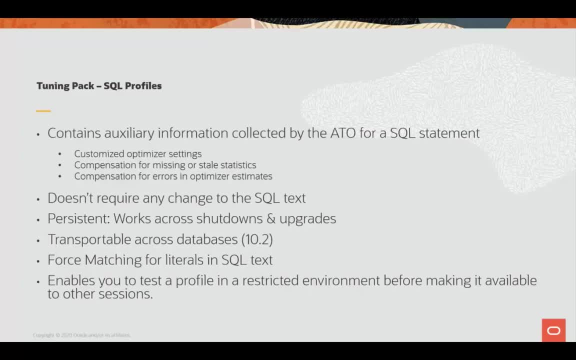 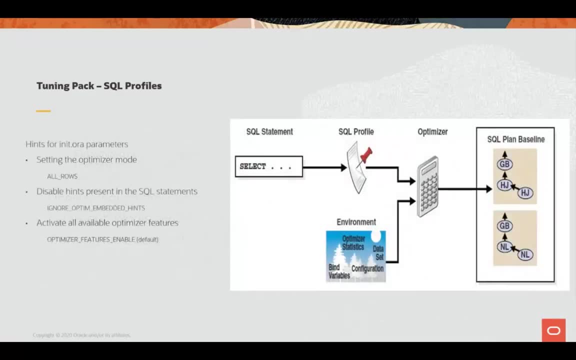 This is really useful to test it out before other sessions can see this SQL profile. So the way it works is: you have the SQL statement, you create the SQL profile that is coming out of the optimizer. The SQL profile is injected inside the optimizer. 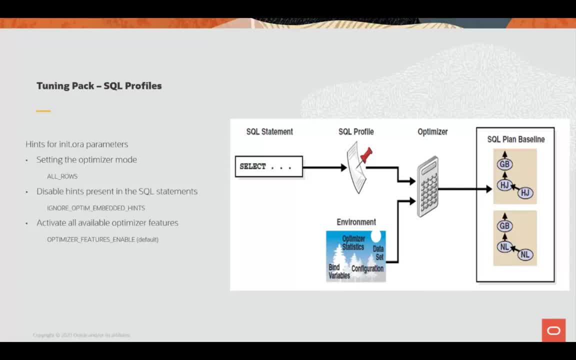 You have environment data like optimizer statistics, bind variables, configuration data sets, So both the SQL profile and all the environment settings are injected inside the optimizer. The optimizer creates the new plans using all the algorithms that it has inside, And then you have the optimizer. 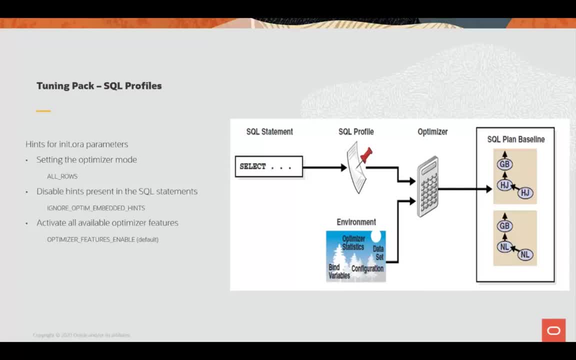 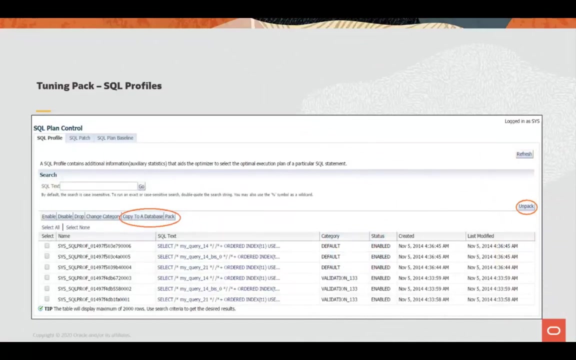 And then, as a best practice, we recommend to use SQL Plan Baseline to create the baseline and lock that plan that is working optimally for that particular SQL statement. If you use Oracle Enterprise Manager, you can go to this specific dashboard that you're. 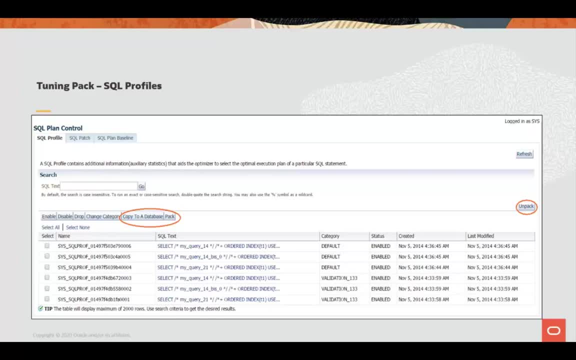 using It's named SQL Plan Control, You can see that we have three tabs. The first one is for SQL profiles. We also have another one for SQL patch and SQL plan baselines. You can manage the full lifecycle of all the SQL profiles in your database. 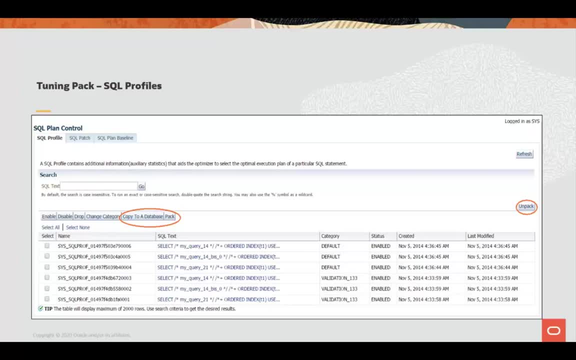 You can see that we're showing you all the available SQL profiles in this particular database. along with the SQL text, Any category, You can see the status, when it was created and when it was modified. You can also use Oracle Enterprise Manager this particular functionality to transfer. 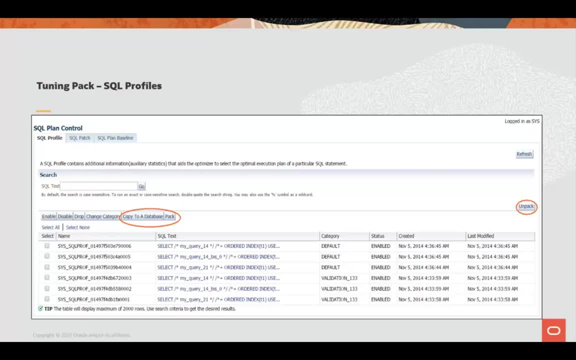 SQL profiles between databases. That goes back to the example that I was telling you. If you create SQL toning sets and you transport the SQL toning set to a test environment, then you can run SQL Toning Advisor, create a SQL profile and then transfer the SQL profile. 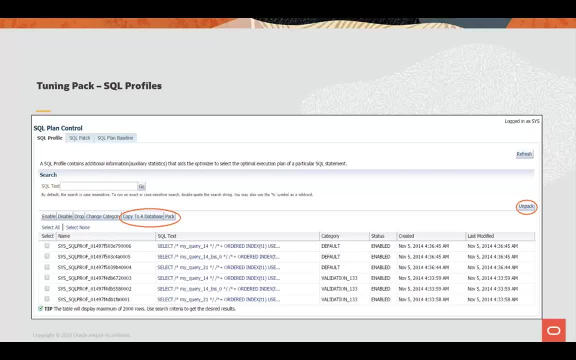 back to your production database, So you run all the APIs. You can run all the APIs. If you have a heavy, heavy workload of running SQL Toning Advisor and testing out everything in the test environment, then you just transfer the result, which is a SQL profile, to your. 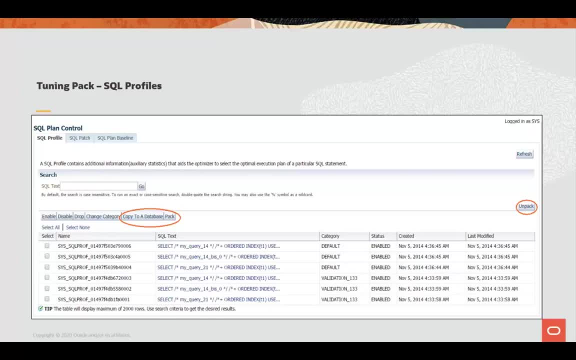 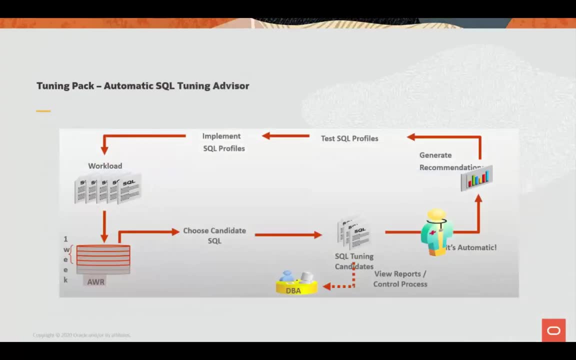 production database when you feel that it's going to generate an optimal plan for that particular SQL statement. We also have the automatic SQL Toning Advisor, So we saw that using SQL Toning Advisor, you can manually call The advisor and start analyzing a SQL statement. 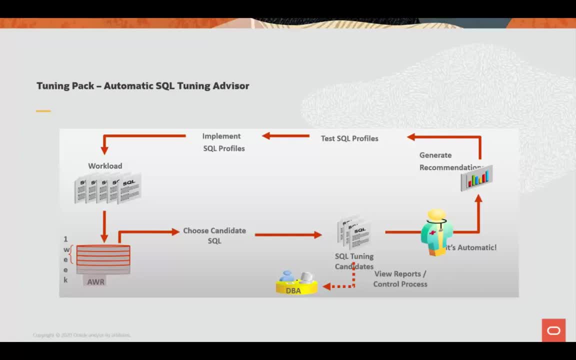 Well, using the automatic SQL Toning Advisor, you can instruct that. you can configure a SQL Toning Advisor to run automatically in your database. So, based on the AWR data that it has, what is going to happen is going to choose a candidate. 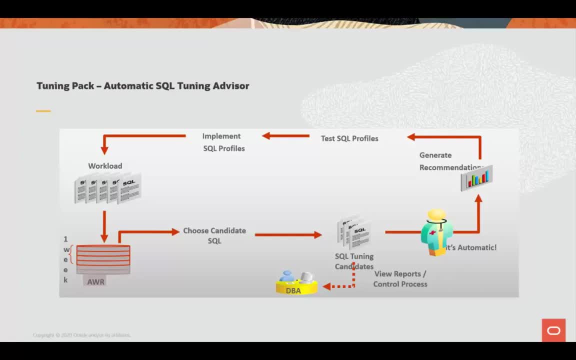 SQL. Then it's going to run SQL Toning Advisor. Then it's going to run SQL Toning Advisor. It's going to generate recommendations for you, It's going to test SQL profiles And, last but not least, if you enable that option, the automatic SQL Toning Advisor can. 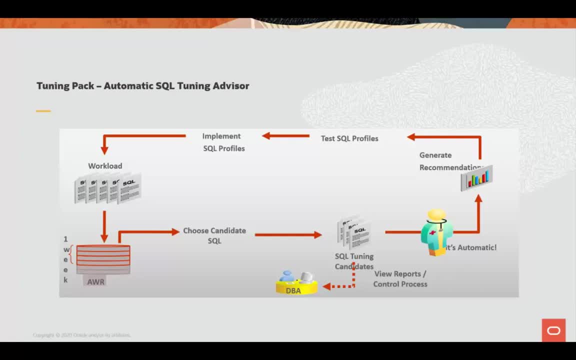 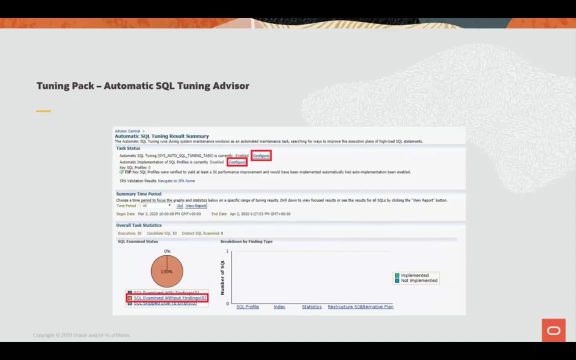 also implement SQL profiles. If not, it will generate a report And it's up to you to go and manually review the report and manually enable those SQL profiles that were recommended. I'm showing you the automatic SQL Toning Configuration. You can see that the task status is set to enable. 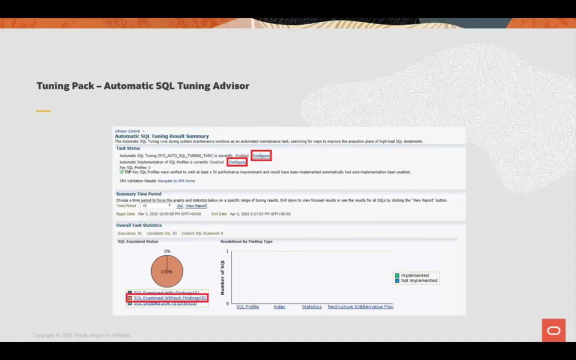 That means that automatic SQL Toning Advisor is going to run automatically, But you can also see that the automatic implementation of SQL profiles is currently disabled. That is by default. This report is showing you the summary in time period. You can see the number of executions. 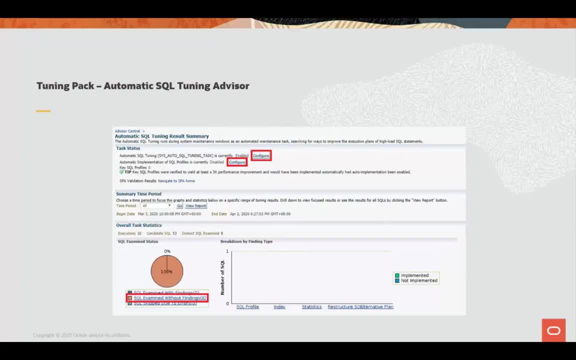 The number of candidates that were identified during the run, the number of distinct SQL examine and also you see how many sequels were found with findings. That means that there is a better execution plan or there is a SQL profile that can be implemented, or 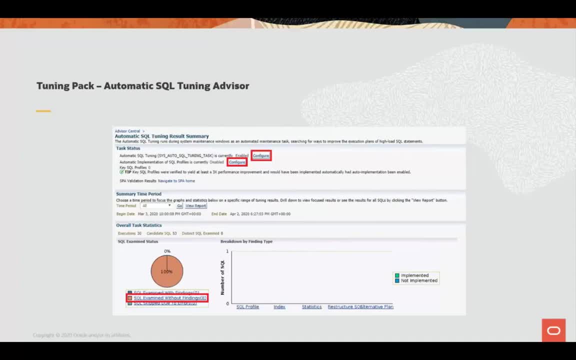 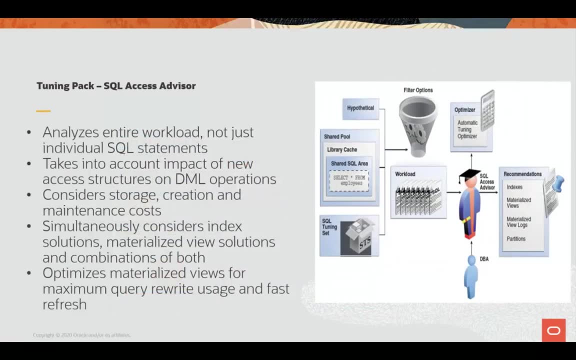 sometimes an index can be a better option for that particular SQL. We also have the SQL Access Advisor, So when we try to create an index or a new structure in our database, we want to make sure that that is the right approach for that particular SQL. That means that this SQL Access 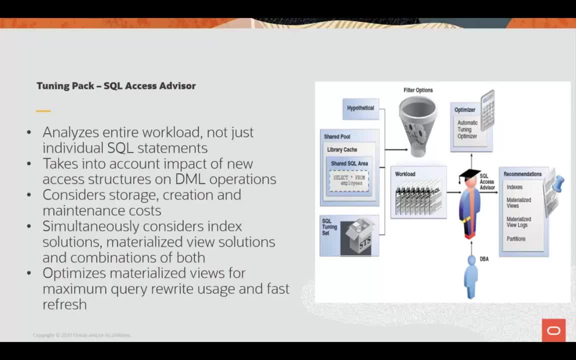 Advisor is going to analyze the entire workload that we have, Not just individual SQL statements. You will take into account the impact of new access structure on DML operations as well. You will consider the storage needed for creation and maintenance costs. You will also consider index solutions or 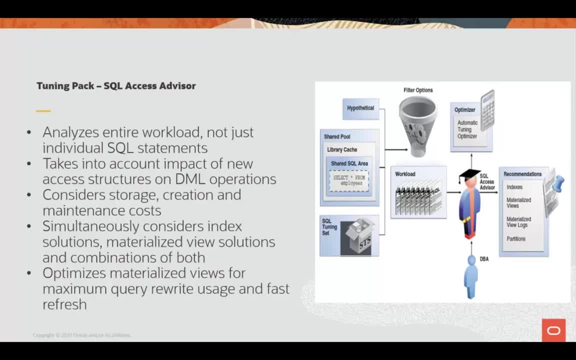 materialized view solutions and or the combination of an index or a materialized view. It will also look like more modern organizations like Amazon that we can Optimize the materialized view for maximum query rewrite using either the standard query rewrite or fast refresh for that materialized view. 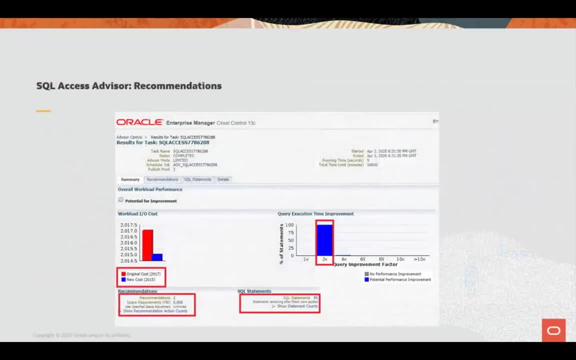 Okay, The way it looks like is. this is an example of a result of a SQL Access Advisor task. On the summary section, you have the overall performance impact for those recommendations. In red you can see the original cost. In blue you see the new cost, which is lower than the original one. 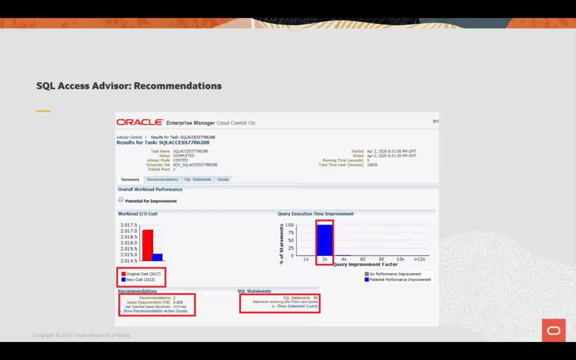 On the bottom of the screen we have the original cost. There are a number of recommendations. We have two of them: The space requirement for the index creation, And on the right side we have the number of SQL statements that were analyzed during that particular session. 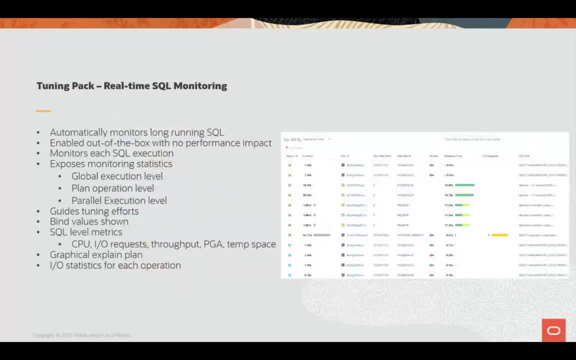 We also have real-time SQL monitoring And real-time SQL monitoring is one of the best features available for this training pack. It will automatically monitor long SQL running statements. So after a specific period of time of the SQL running, real-time SQL monitoring is going to pick up the SQL statement. It's going to show you that SQL statement inside the SQL monitoring screen. 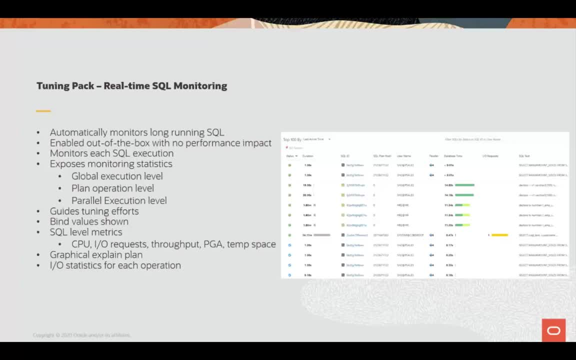 It's enabled out of the box. There's no performance impact on enabling this. It will monitor each SQL execution and it will expose several monitoring statistics, Like the global execution level, plan operation level and parallel execution level. You can see that we have the status, we have the duration, the SQL ID, the SQL plan hash value, the user name and the PDB that it's running on- if there is any degree of parallelism, the database time that it took for each of the executions, the IO requests and the SQL text. 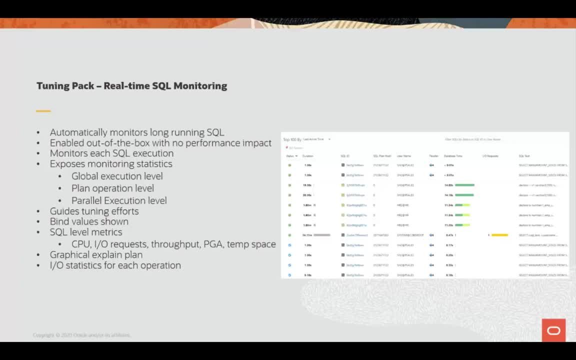 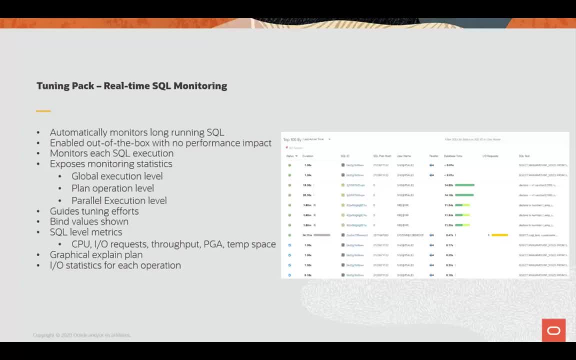 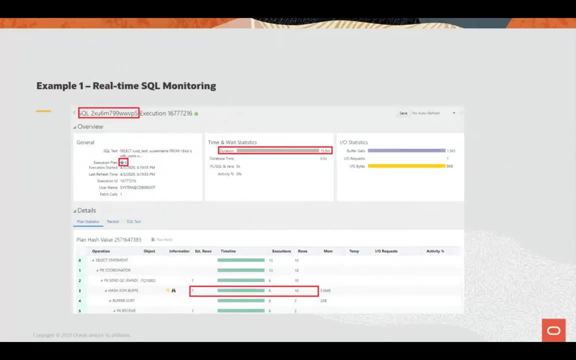 And, as I mentioned, we have IO statistics for each operation. This is an example of how a real-time SQL monitoring page looks like for a specific SQL ID. I'm highlighting information about the SQL ID If the SQL is running on any parallel. 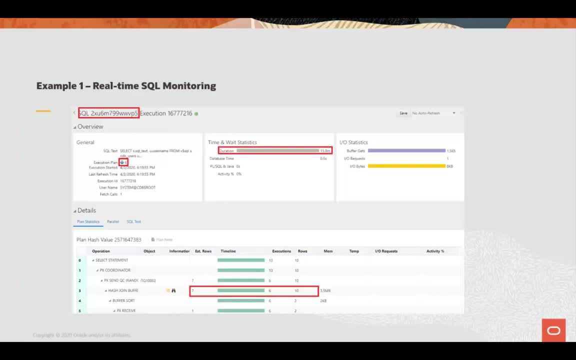 we can see that we have six of them any time- and weight statistics, the duration and also details of the execution plan. right, We have the select statement, then we have the parallel coordinator, the slave coordinator of the parallel query. We have, on the row number three, the hash join buffer. 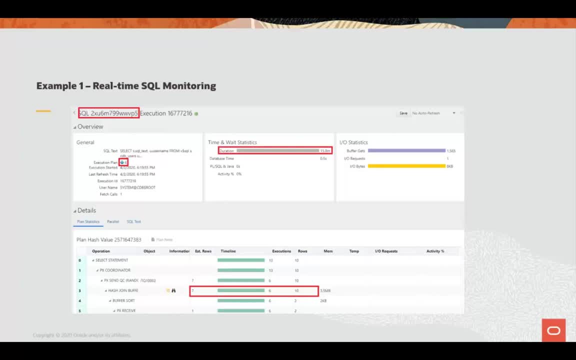 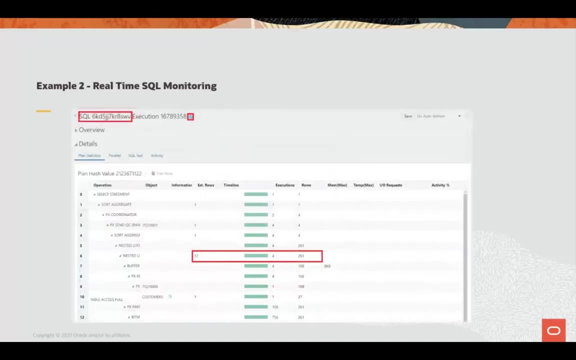 And here clearly you can see that the optimizer was estimating seven rows, but the actual number of rows were 10.. So there's a mismatch over there in the estimation of the cardinality of this specific SQL ID. Here's another example where we have the SQL ID, the execution ID. 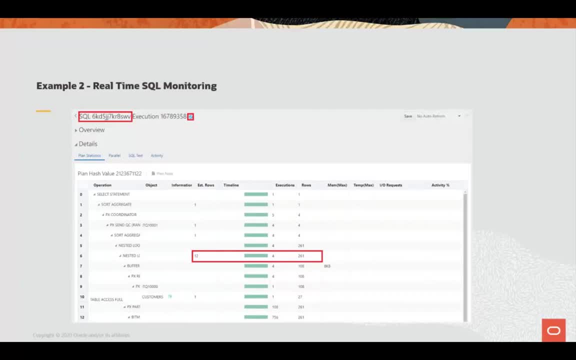 and also there is a nested loop on row number six. You can clearly see that we have an estimated rows of 12 by the optimizer, but the actual number of rows were 261.. This is a clear indication that we should probably gather statistics on this specific SQL. 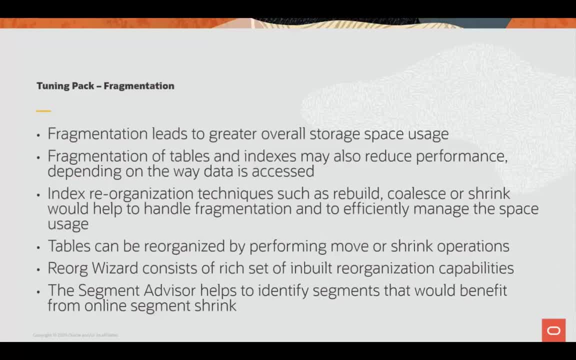 Last but not least, let's talk about fragmentation, And we know that as the data is changing inside our segments. right, We have deletes, inserts, updates. This can lead to a greater overall storage space usage. right, We can have fragmentation of tables and indexes. 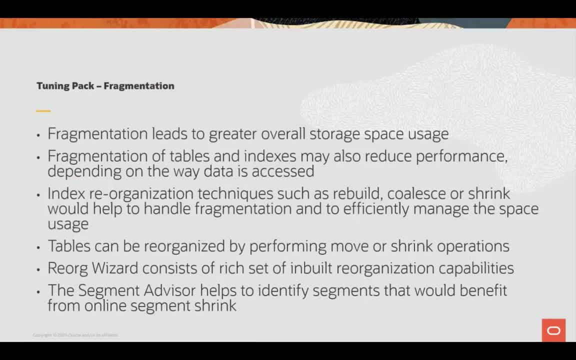 This could reduce the performance depending on the way we're accessing the data right. So we can reorganize indexes using techniques such as rebuild, We can shrink right. We can also reorganize tables using move or shrink operations And we have the segment advisor. 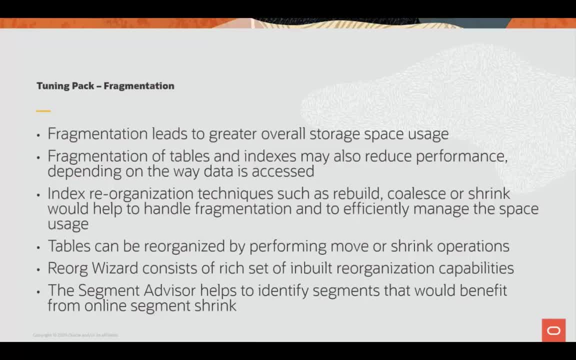 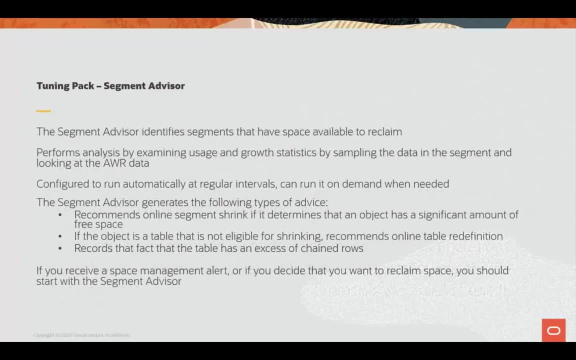 That can help you to identify those segments that will have a benefit from that online segment shrink. This segment advisor is going to identify these segments And it's going to give you information about how much space is available to reclaim. You will perform this analysis by examining this usage and grow the statistics. 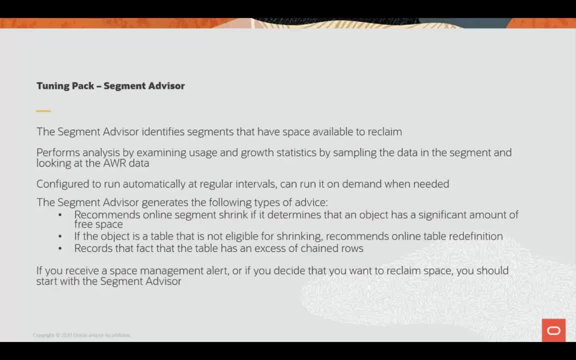 by also sampling the data in the segment, but also looking at the data in the AWS repository. This is configured to run automatically at regular intervals. You can modify this configuration as well. It will generate different types of advice. You will recommend online segment shrink. 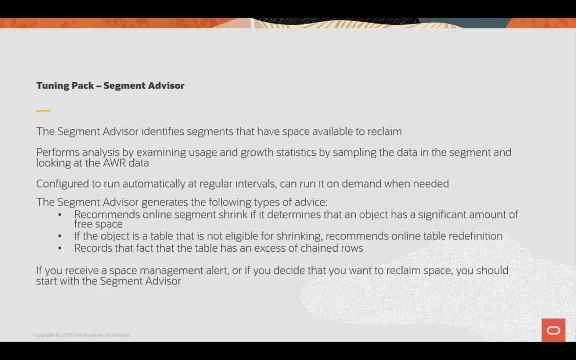 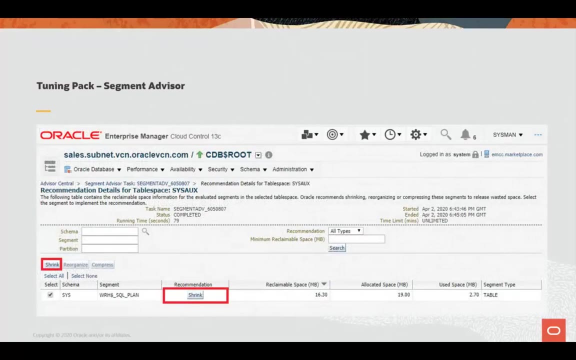 It will tell you if the object is a table or if it's not eligible for shrinking, And it also going to record that the table has an excess of change rows. If that's the case, right, the way it looks like is: this is an output of the recommendation report. 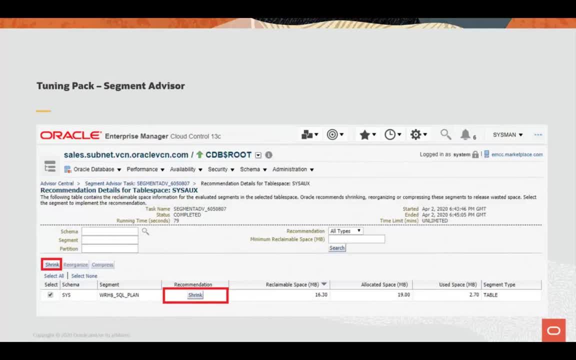 from the segment advisor. we have a table here that the recommendation is to shrink. we can reclaim around 16 megabytes for this particular table. you can see that the total allocated space is 19 megabytes. that means that this table is only using 2.7 megabytes. right, this is a table type. last but not least, 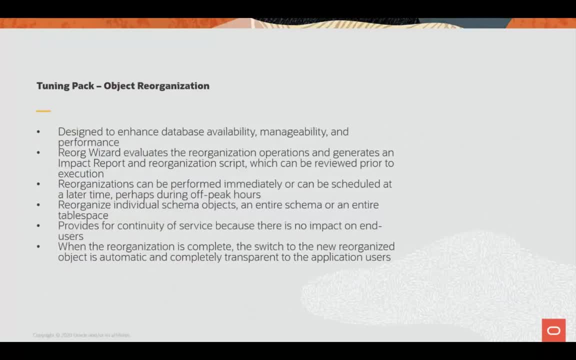 we have object reorganization and this is designed to enhance database availability. right, we have our reorganized wizard that is going to evaluate the reorganization operations and it's going to generate an impact report. right, this reorganization can be performed immediately or you can schedule that for a later time, perhaps. 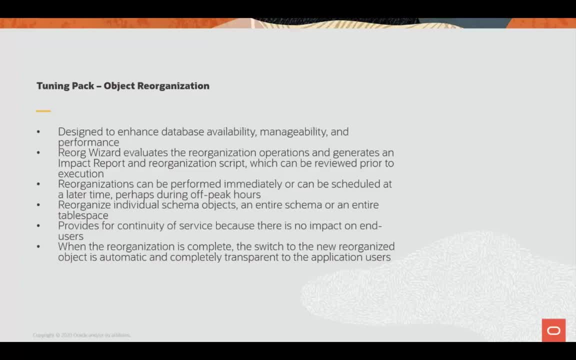 during off-peak hours. it's going to reorganize individual schema objects or the entire schema. if you instruct the the reorg wizard to do that provides continuity of service because there is no impact on end-users, and when the reorg is complete it's going to switch to the new reorganized object. 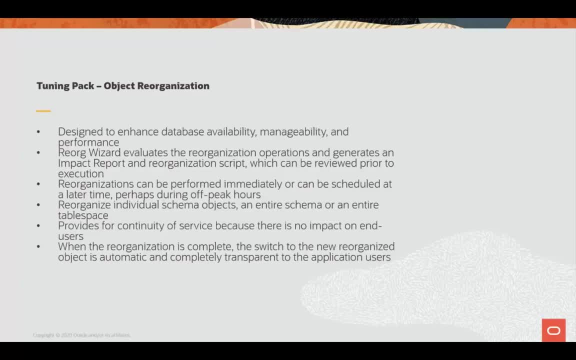 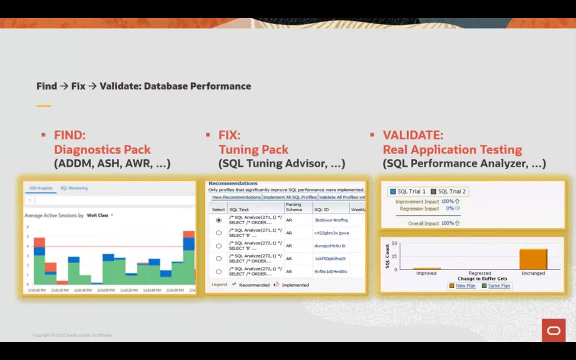 automatically and then it will be able to inform that the new, reorganized object and it's completely transparent to the application users. in summary, what we saw today is that we have defined- I explained- the Diagnostics Pack, all the data that we're gathering inside AWR, how we make use of this data right to. 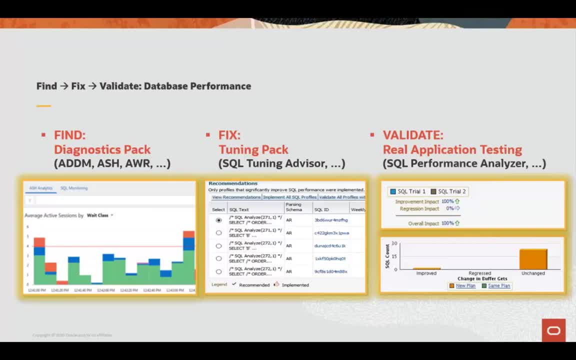 identify issues. so we find issues using the Diagnostics Pack. we also have the fix, which is the Toning Pack. we went through the SQL Toning Advisor and all the advisors that we have available in order to fix problems that were identified using the Diagnostics Pack. the last step is to use real application. 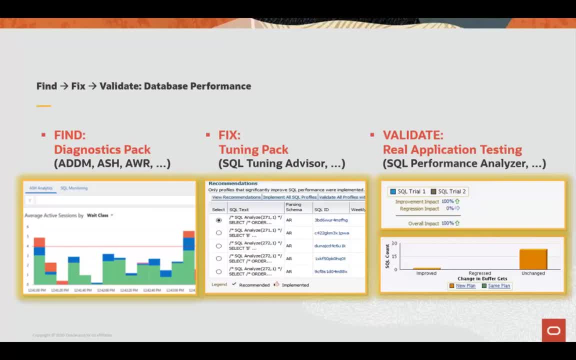 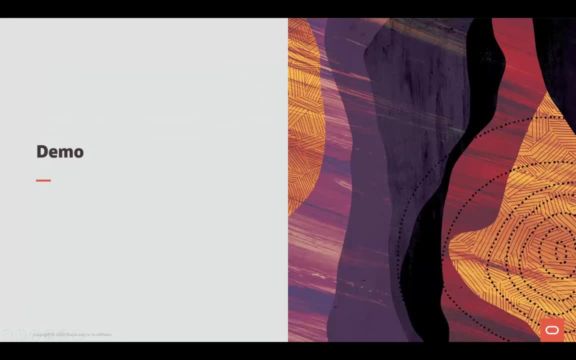 testing, which is a third and additional database pack in order to validate issues using SQL Performance Analyzer. but now let's jump into a quick demo where I show you how to identify a SQL statement that is performing using a suboptimal plan, and how we can identify it and then tune it using SQL Toning Advisor. 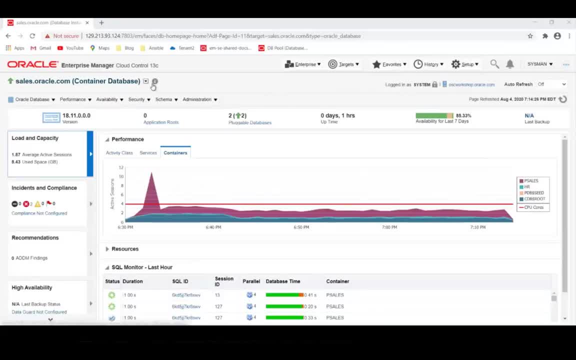 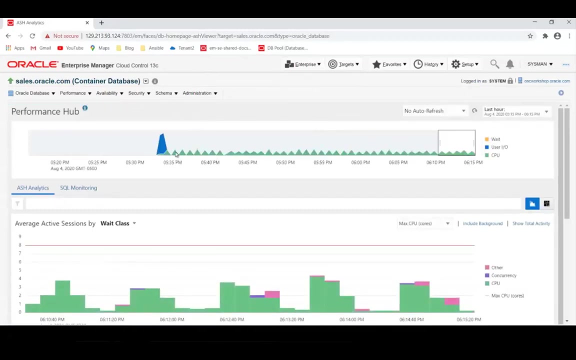 okay, here I have a test database where I have some workload running. I'll click on performance, then I'll click performance hub and click ask analytics. remember that we were discussing about active session history. right the page is bringing up the top graph where it is providing information about the current active active sessions in the database. 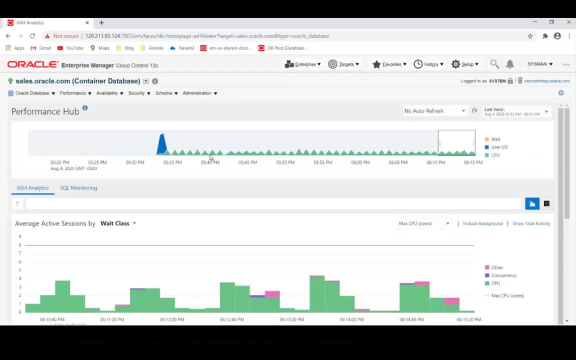 and also we can see different colors in the graph. you can see on the right side that the the green part represents the CPU utilization. then we have the user IO and also we have wait activity for those sessions. I scroll down and I have performance information. 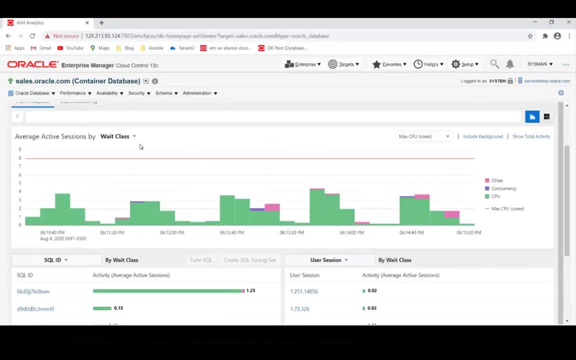 related to the average active sessions. this is filtered by wait class. I can filter them by different dimensions. I have wait class, wait event instance service module. on the SQL side I have SQL ID, the top level SQL ID, SQL plan, hash value for PL SQL as well. I can filter by PL. 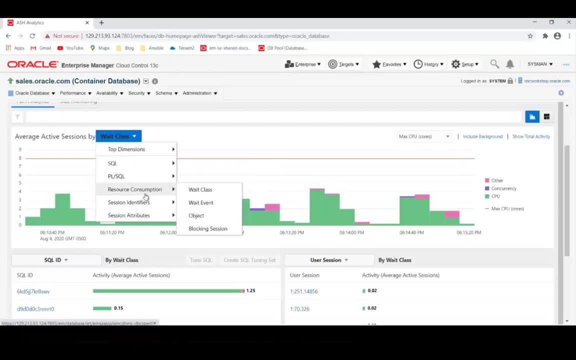 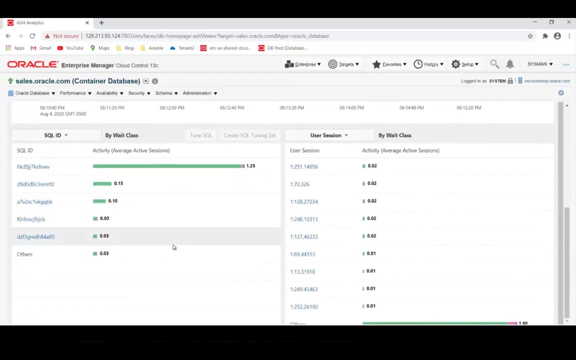 SQL or the top level PL SQL resource consumption. consumption the weight class. this is the one that I have right now: weight, event, object or blocking session. if I keep scrolling down, then on the right side I have information about the SQL statements running in that particular time frame. 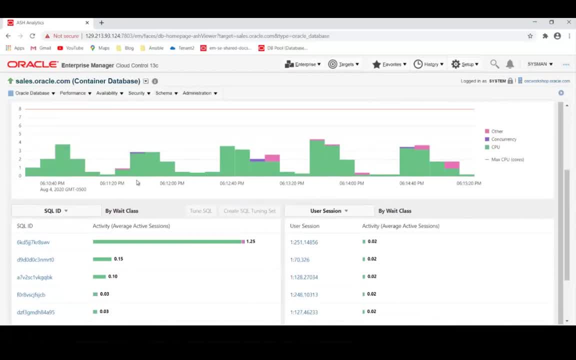 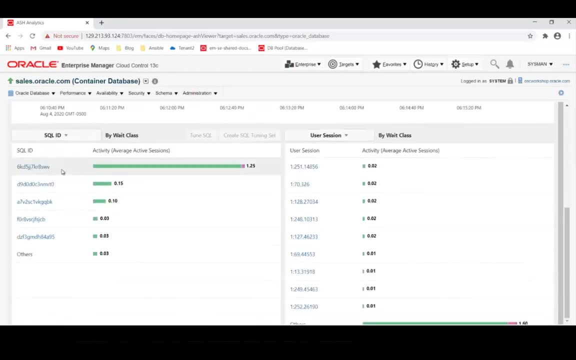 right, which in this case is five minutes, from 6: 10 to 6: 15.. I also can see that this is ordered by the amount of resources that the, the SQL ID, is consuming, so the top one is is the one that is consuming more CPU we have. 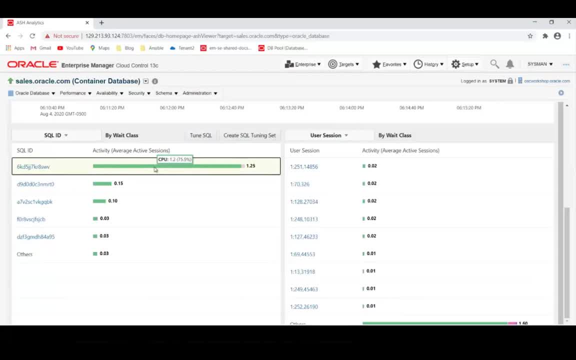 1.2, which accounts for 75 percent of the CPU use usage in the database, and on the right side I have the sessions that belong to these particular SQL IDs that I have. so, making use of AWR data data that the database is collecting, I'm 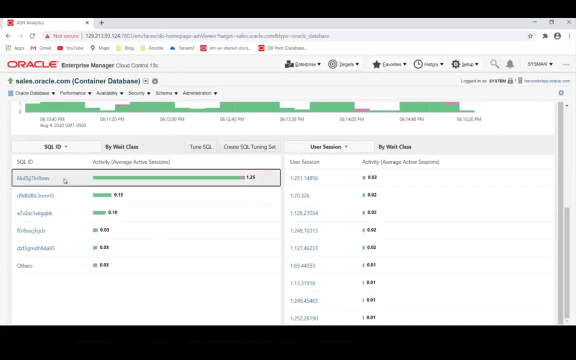 able to identify the top offenders right? I have this six kd d90 a7v SQL ids right, so I'm going to click on the first one. I highlight that row and you can see that right away. I have the option to create a SQL telling set. We already discussed what a SQL tuning set is and also I can invoke the SQL Tuning. 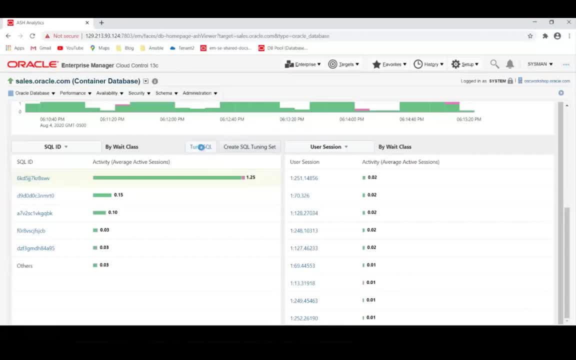 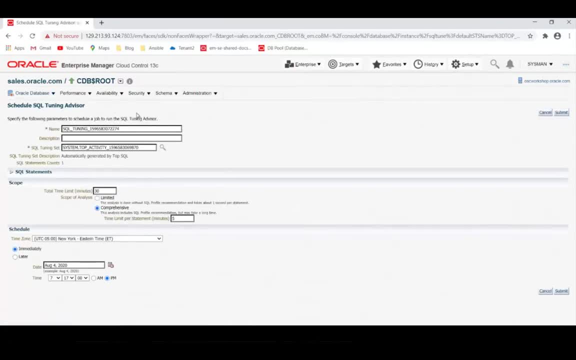 Advisor by clicking TuneSQL. I'm going to click on that. SQL Tuning Advisor page comes up. I have a couple of preset inputs like: the name of the task is creating a SQL Tuning Set for me that has one SQL statement. of course I can expand the SQL statements and 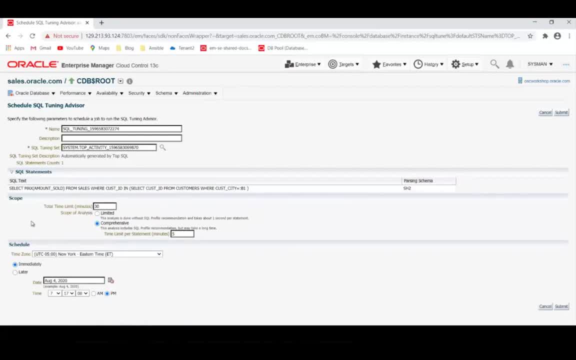 also the scope. Remember that I explained during the presentation that by default we have five minutes per SQL statement. I'm just going to leave the default and then I can schedule this task. I can run that immediately or also instruct SQL Tuning Advisor to run. 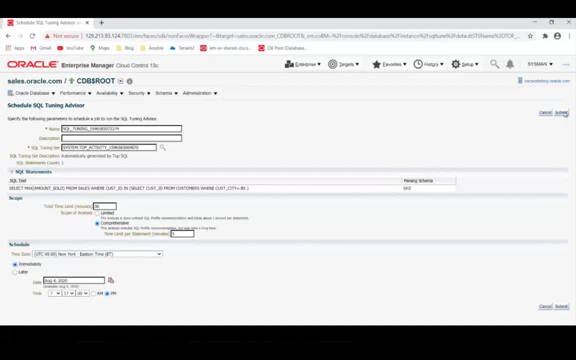 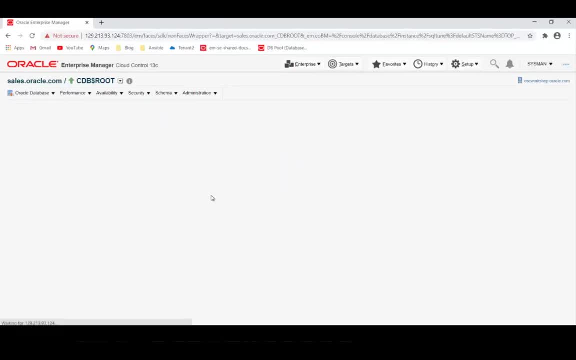 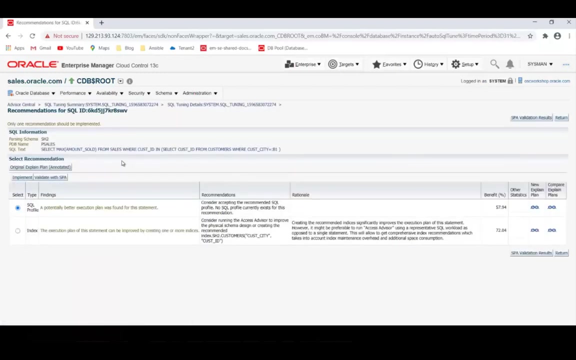 later I'll click submit. I want to run that right now And this task won't take more than 20, 25 seconds to complete. It's just one small SQL statement. Okay, Completed. So these are the recommendations. create a SQL profile or create. 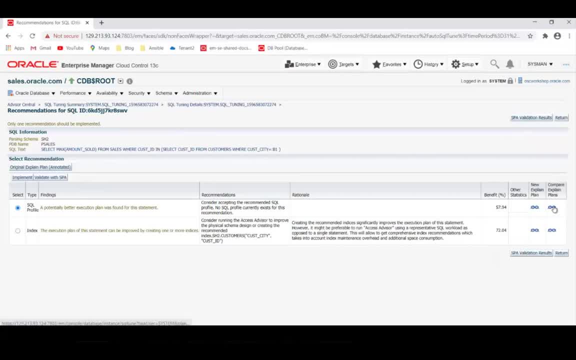 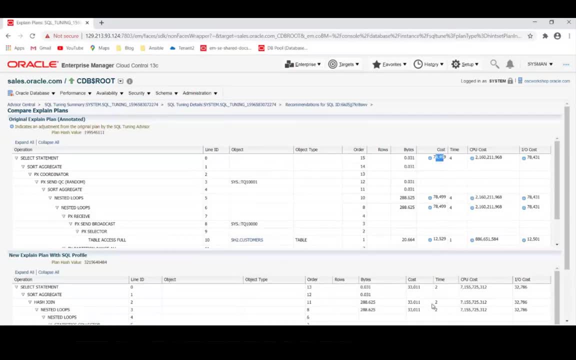 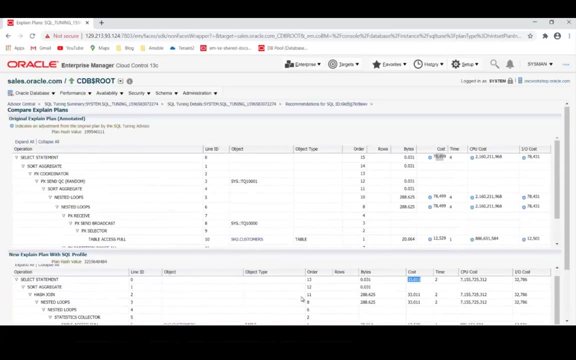 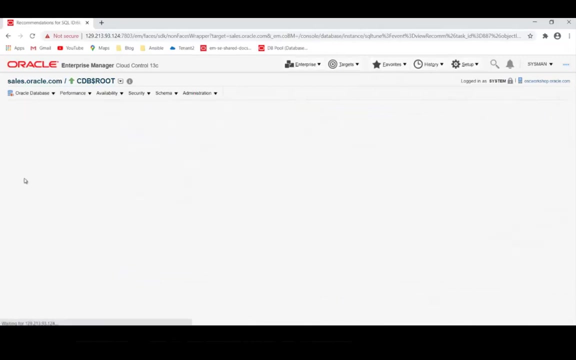 an index. We also can compare the explained plans. I'm going to click on that. The difference between the cost of the original one compared with the cost of the new explained plan. If we implement the SQL profile. go back to recommendations, Select this one and I'm going to click implement. Okay, I can force the SQL Profile implementation. with the force matching signature of the sequel. In this case I have by and by all the time. in terms of this cycle, I can give it two options. The first option is to send to the SQL profile, and the second option is to send a target to the SQL profile. So then I can. 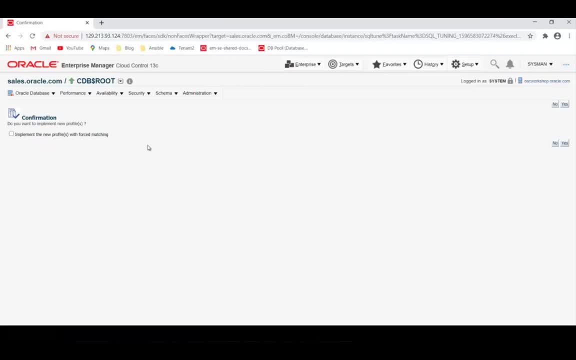 send that request to the SQL profile and then I can see the request that the client has. This is the most flexible process for me. I can send a request to the SQL profile and I can, so I'm not going to select that, I'm gonna click yes, I want to implement that. 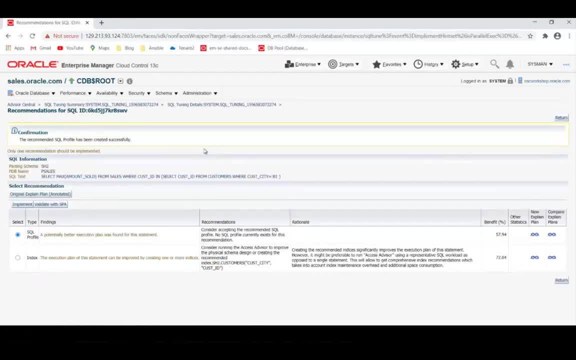 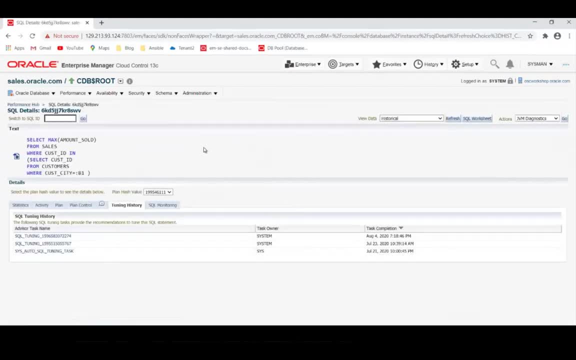 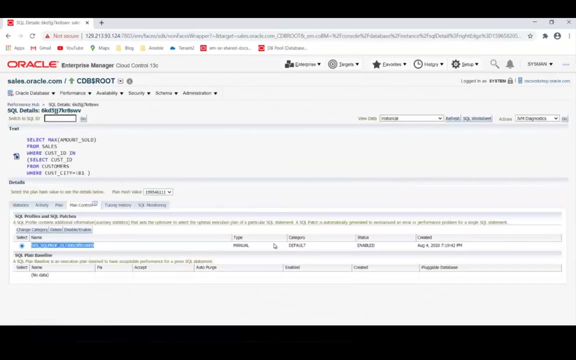 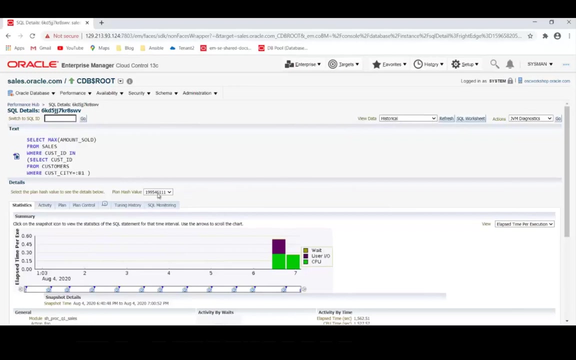 SQL profile and that SQL profile was successfully created. I can go back to the SQL statement stats. if I click on plan control, you can see that I have the new SQL profile. it was, it was created manually, it's enabled and the time that it was created. in statistics I can see the historical statistics of that SQL. 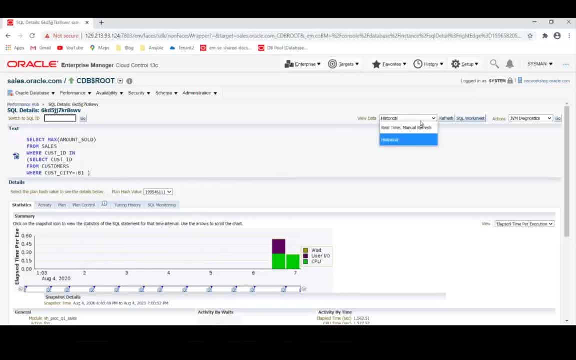 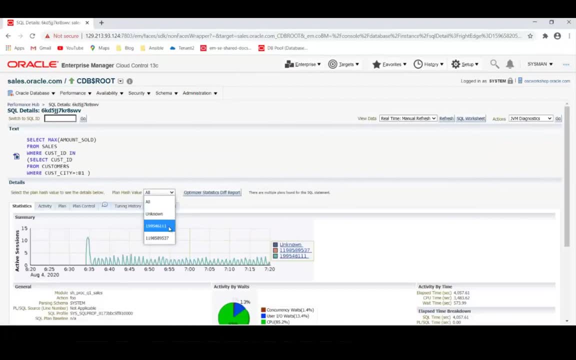 statement. this is the original plan hash value. click manual refresh. okay, you can see. now I have two SQL to plan hash values for that particular sequel: the original one, which is the one nine nine five and the new one that was created, that is 1198. you can see that as soon as we created the SQL profile. now. 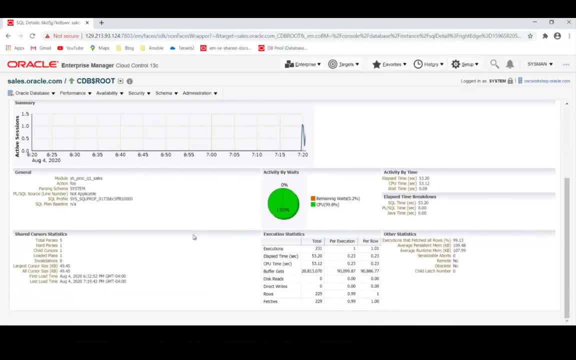 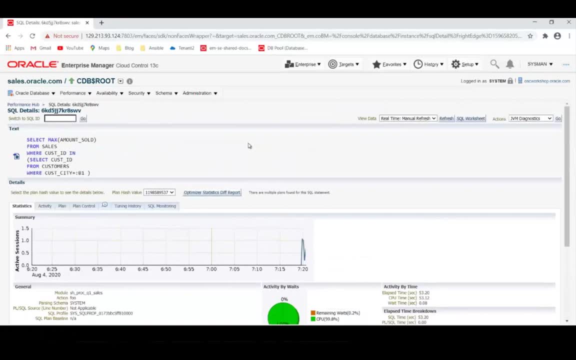 the new execution plan is up and I have the new execution statistics for that particular SQL ID. okay, so we cover doing this small demo: how to make use of AWR data data that the database is collecting using the diagnostics pack. I'm also using the SQL turning pack and the SQL turning advisor, which is a tool. 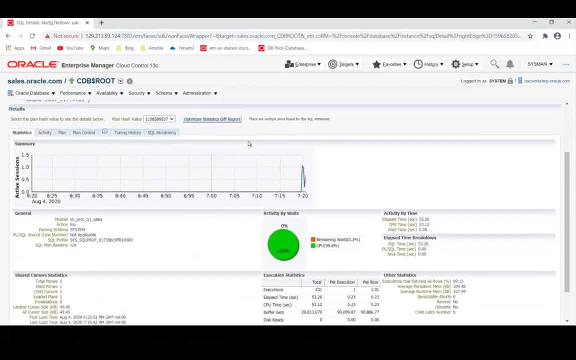 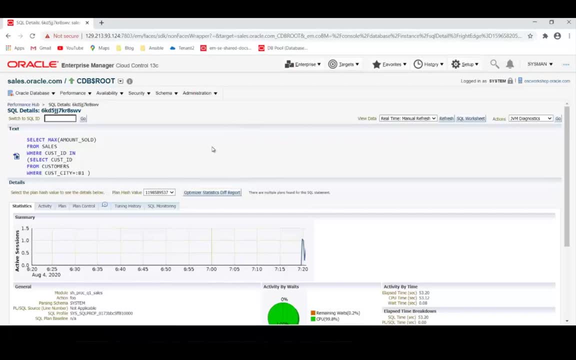 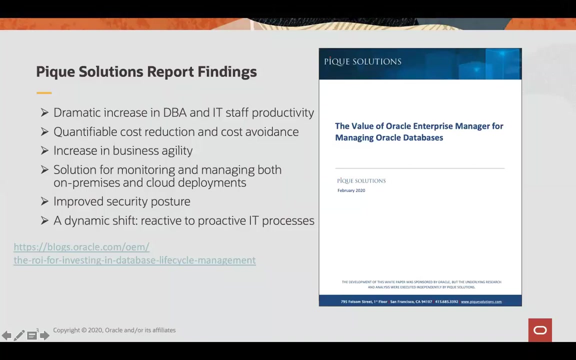 inside the SQL turning pack in order to fix that particular SQL statement. so, Tim, this concludes my presentation, the webinar on the technical side. let me know if you have any questions from our attendees. all right, thank you, Alfredo. that was a great presentation, actually a great demonstration of moving from diagnostics with performance hub into SQL tunings. 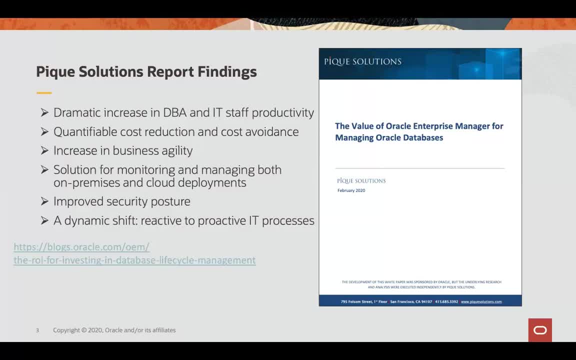 tuning pack. so that was fantastic. thank you very nicely done so. peak solutions wrote a report for us. it's really well researched. they did some extensive, deep interviews with many of our customers, put together a real quantifiable report showing cost reductions, cost avoidance and the biggest thing probably was around the dramatic increase in DBA and 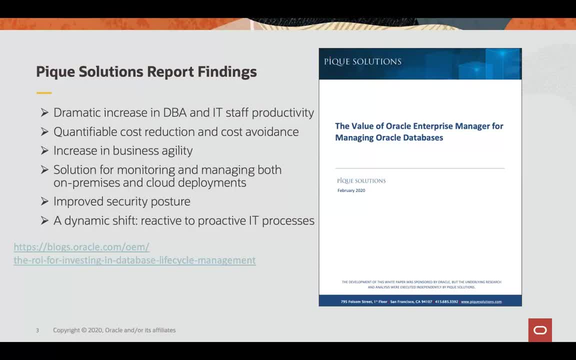 IT staff productivity. so if you're looking to invest in doing some of these activities with enterprise manager, this is a great report to help justify some of that. so take a look at the link below. and we do have our webcast series. we have some upcoming events you can see on the 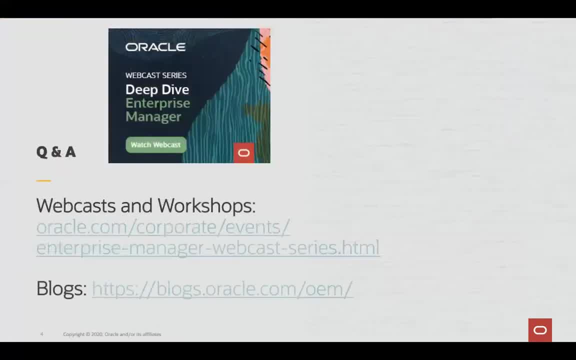 calendar there, as well as many of our previous webcasts on demand. we are planning to post some workshops as well, so stay tuned for that as well, and those be coming soon. the blogs are down on the bottom that. we have some really good technical blogs, announcements and other assessments that you'll see in our blogs. 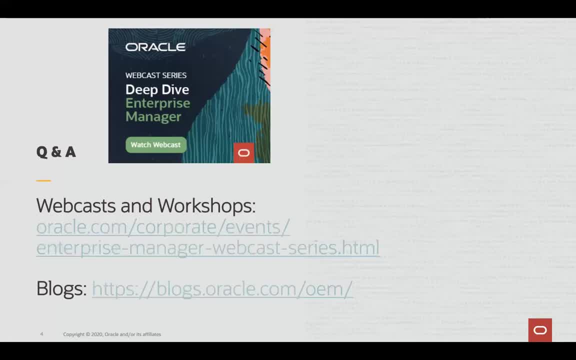 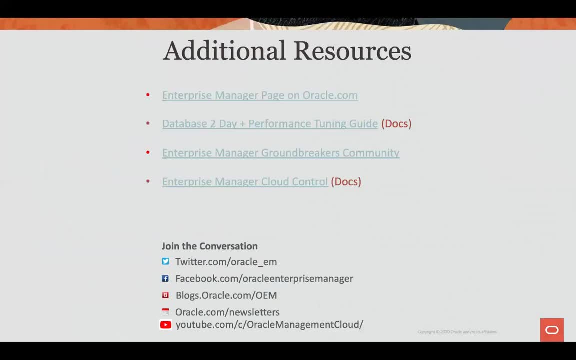 you can visit our website and join in the conversation. we have quite a presence on Twitter. we have a big community that slash Oracle, underscore, EM and then down on the bottom, we do have a very fleshed out YouTube channel, so take a look at some of the videos of demonstrations, of presentations and so on on our YouTube. 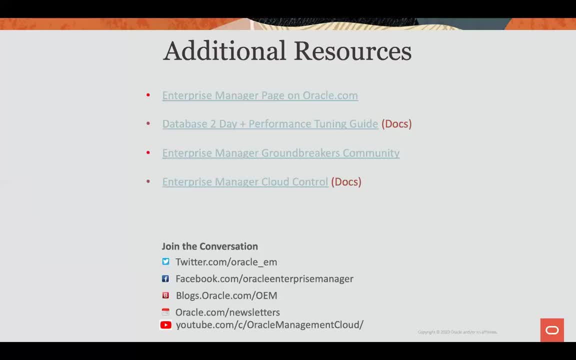 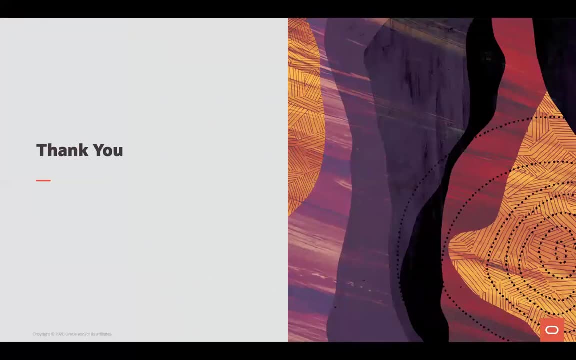 channel. all right, thank you very much, all of you, for attendance, thank you for your attention and thank you for joining us on the webinar. we'll see you at the next one. questions and participation. Really appreciate that, Alfredo. great job on the presentation and